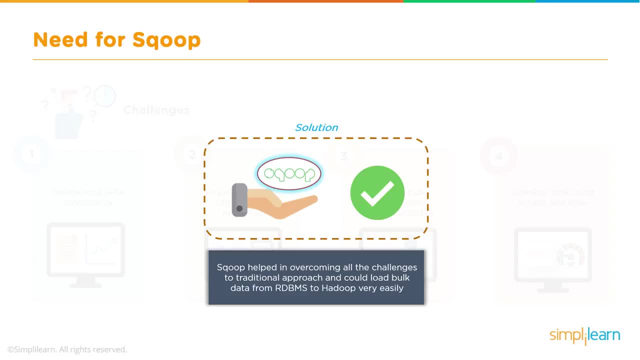 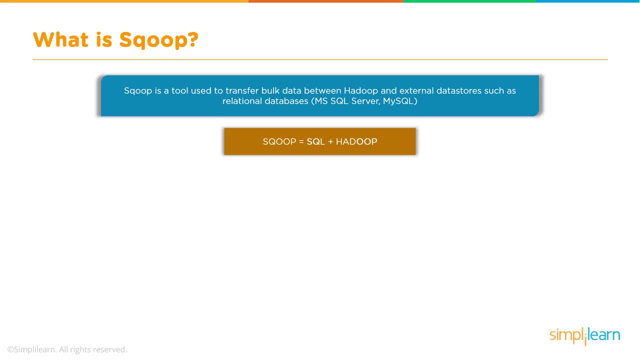 SQL and you wanna bring that data into your Hadoop warehouse, your data filing system, And that's where Scoop comes in. So what exactly is Scoop? Scoop is a tool used to transfer bulk of data between Hadoop and external data stores. So it's has relational databases And 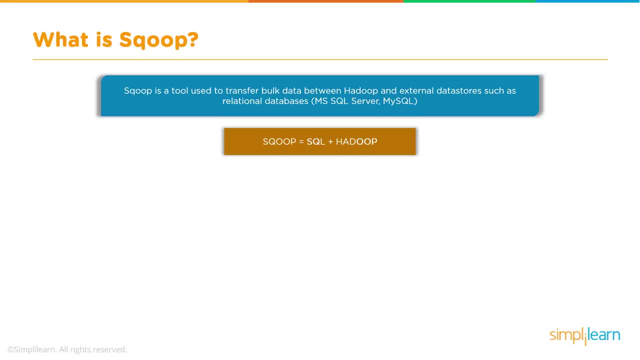 MySQL server or ah, the Microsoft SQL server or MySQL server SQL Server. So Scoop equals SQL plus Hadoop SQL Server, Because Hadoop was very SQL Server. So Scoop equals Sql SQL Server. So Scoop equals SQL plus Sql. 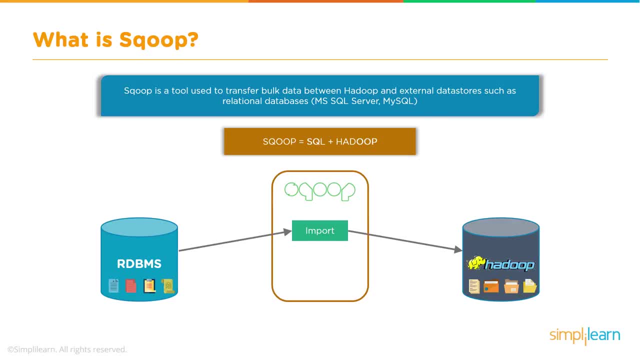 Hadoop and you can see here we have our RDBMS, all the data we have stored on there, and then your scoop is the middle ground and brings the import into the Hadoop file system. it also is one of the features that goes out and grabs the 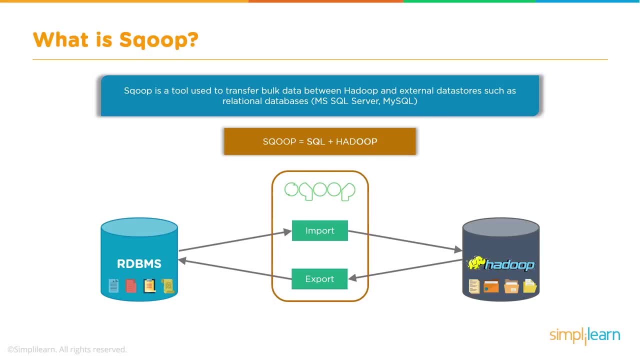 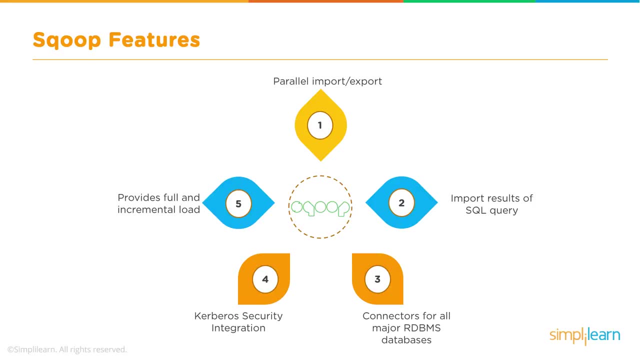 data from Hadoop and exports it back out into an RDBMS. let's take a look at scoop features. scoop features has parallel import and export as import results of SQL query connectors for all major RDBMS databases. Kerberos security integration provides full and incremental load. so we look at parallel. 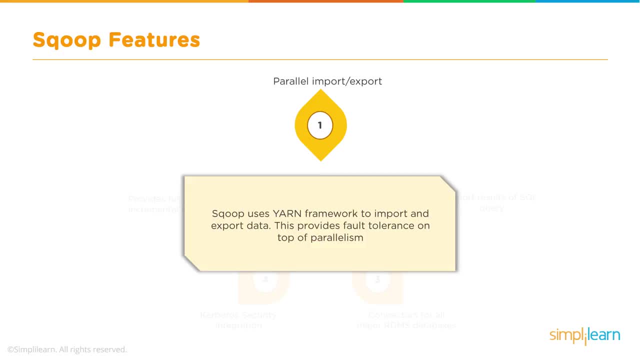 import and export scoop uses yarn, yet another resource negotiator framework, to import and export data. this provides fault tolerance on a top of parallelism. scoop allows us to import the result returned from an SQL carry into the Hadoop file system or the HDFS, and you can see here where the import results of 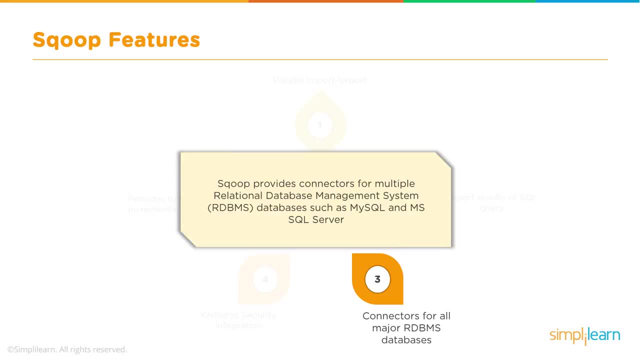 SQL query come in. scoop provides connectors for multiple relational database management system RDBMS databases such as my SQL and Microsoft SQL server, and has connectors for all major RDBMS databases. scoop supports Kerberos computer network authentication protocol that allows nodes communicating over a non secure network to prove their 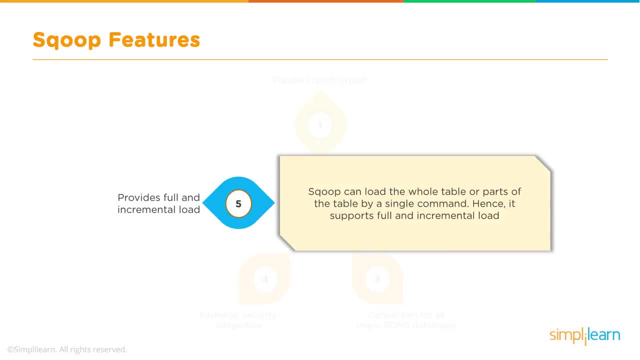 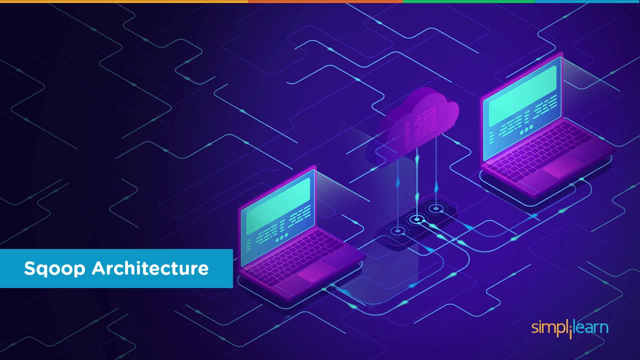 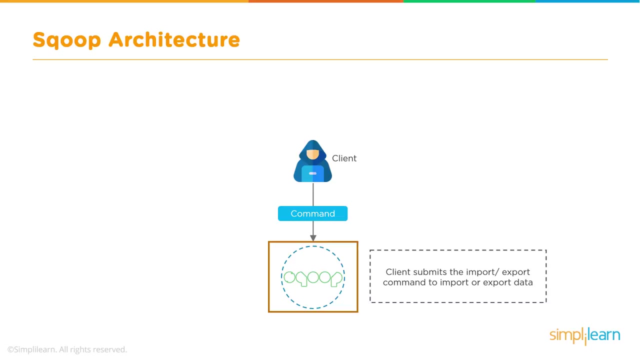 identity to one another in a secure manner. scoop can load the whole table or parts of the table by a single command. hence it supports full and incremental load. let's dig a little deeper into the scoop architecture. we have our client- in this case a hooded wizard- behind his laptop. you never know who's going to be. 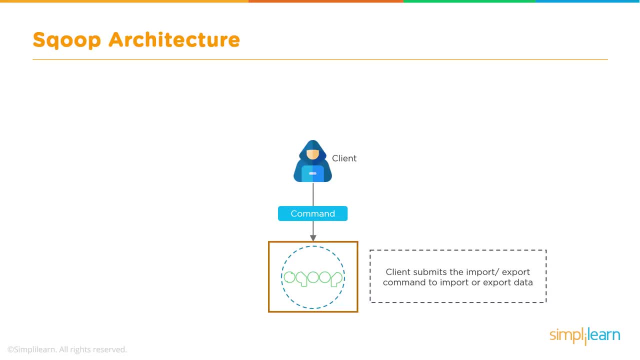 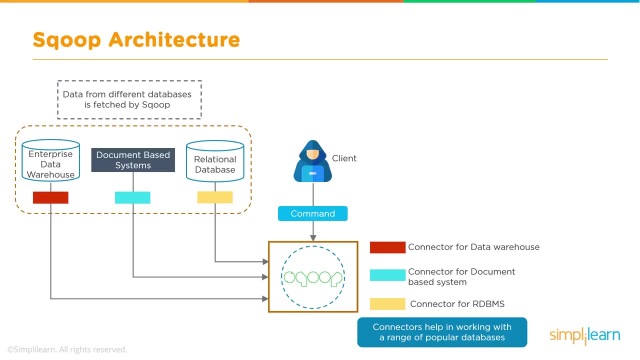 accessing the Hadoop cluster and the client comes in and sends their command, which goes into scoop. the client submits the import export command to import or export data. data from different databases is fetched by scoop and so we ever enter enterprise data warehouse document based systems you have connect. 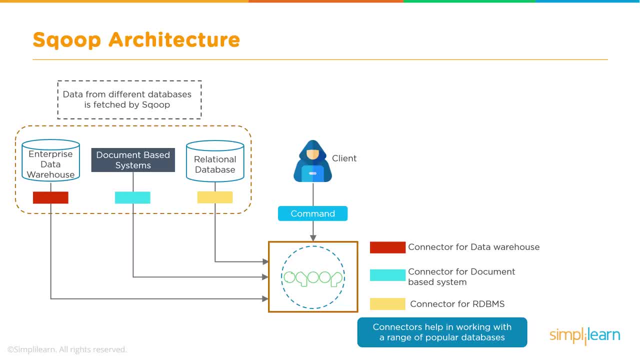 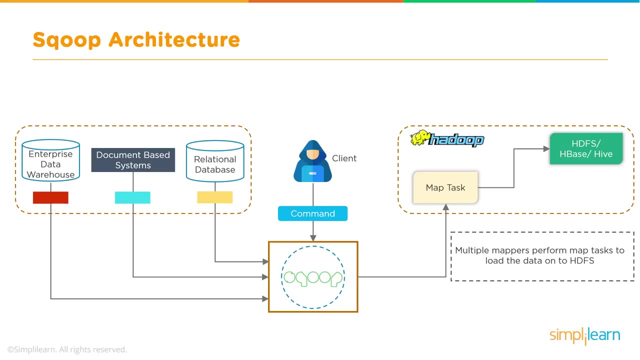 connector for your data warehouse, a connector for document based systems which reaches out to those two entities, and we have our connector for the RDBMS. so connectors help in working with a range of popular databases. multiple mappers perform map tasks to load the data onto HDFS, the Hadoop file system, and 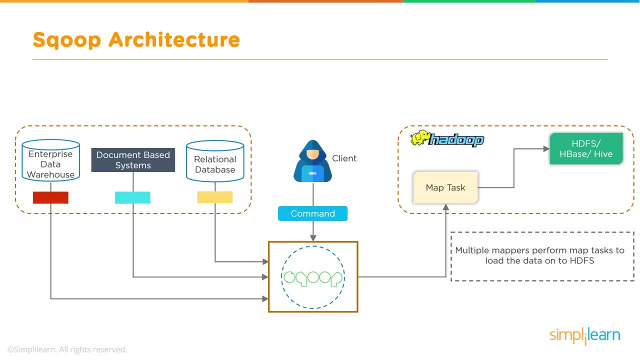 you can see, here we have the map task. if you remember from Hadoop, Hadoop is based on map reduce, because we're not reducing the data, we're just mapping it over. it only accesses the mappers and it opens up multiple mappers to do parallel. 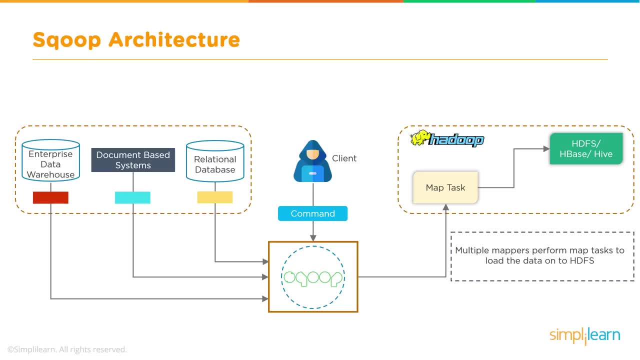 processing and you can see here the HDFS HBase Hive is where the target is for this particular one. similarly, multiple map test will export the data from HDFS on to RDBMS using scoop export command. so just like you can import it, you can now export it. 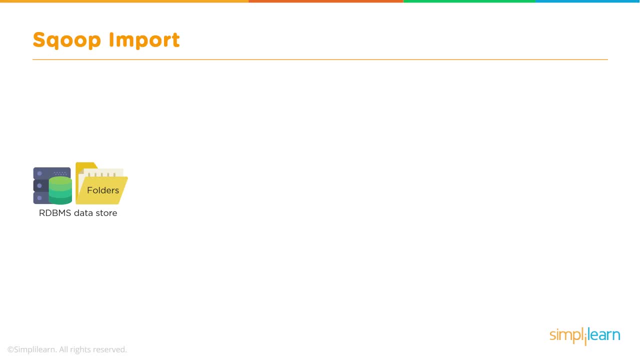 using the multiple map routines, scoop import. so here we have RDBMS data store. we have the folders on there. so maybe it's your company's database, maybe it's an archive at Google, with all the searches going on. whatever it is, usually you think with scoop, you think SQL, you think my sequel server or Microsoft SQL. 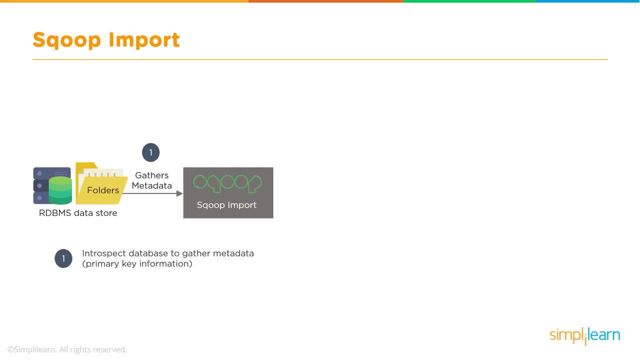 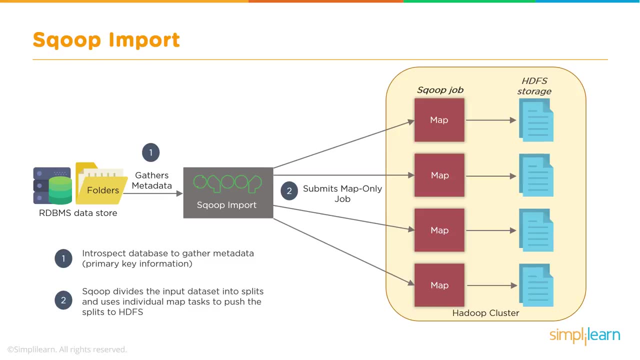 server, that kind of set up so it gathers the metadata and you see the scoop: import, so introspect database to gather metadata, primary key information, and then it submits. so you can see: submits map only job. remember we talked about map reduce. it only needs the map side of it because we're not reducing. 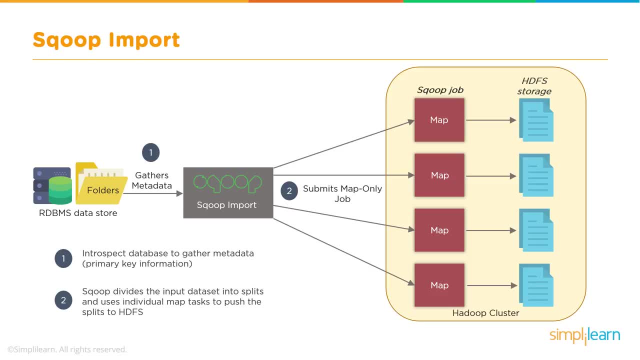 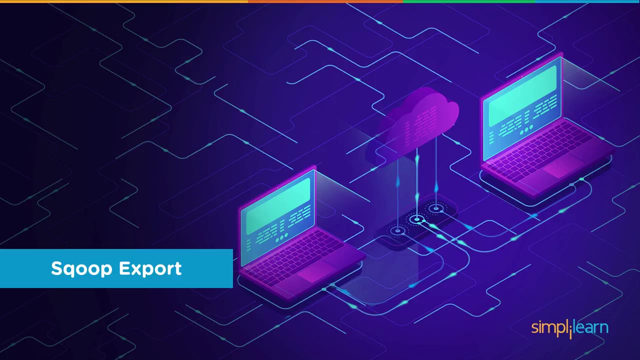 the data. we're just mapping it over. scoop divides the input data set into splits and uses individual map tests to push the splits into HDFS, so right into the Hadoop file system. and you can see down on the right is kind of a small depiction of a Hadoop cluster. and then you have scoop export. so we're gonna go. 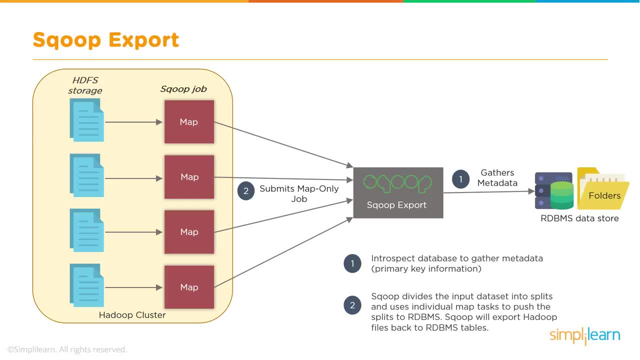 the other direction and with the other direction you have your Hadoop file system storage, which is your Hadoop cluster. you have your scoop job and each one of those clusters then gets a map mapper comes out to each one of the computers that has data on it. so the first step is you've got to gather the 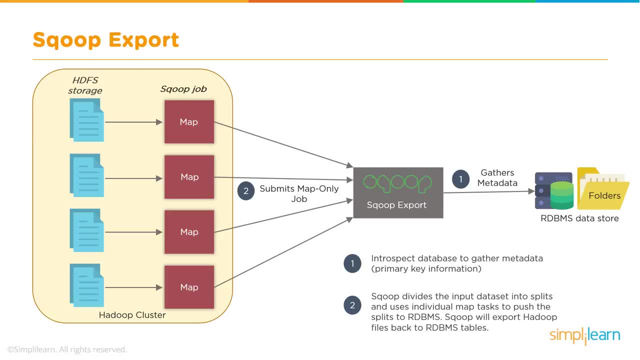 metadata. so step one, you gather the metadata. step two submits map only job introspect database to gather metadata- primary key information. scoop divides the input data set into splits and uses individual map tests to push the splits to RDBMS. scoop will export Hadoop files back to RDBMS tables. 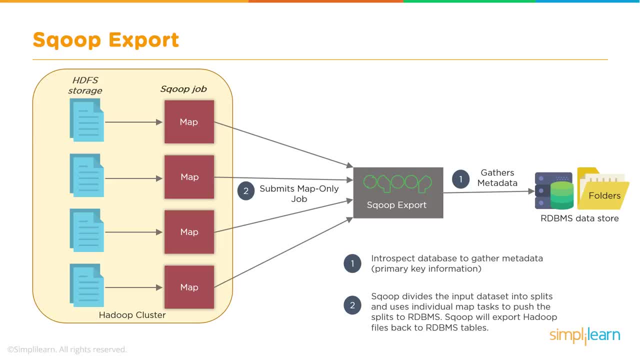 you can think of this in a number of different manners. one of them would be if you're restoring a backup from the Hadoop file system into your enterprise machines. there's certainly many others. as far as exploring data and data science, so as we dig a little deeper into scoop, input we have, our connect are JDBC in. 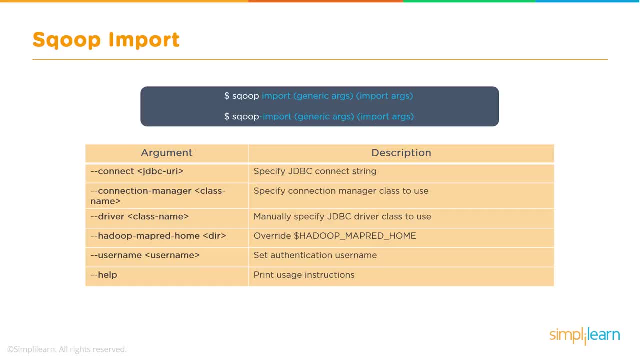 our URL so specified the JDBC connect string Connecting Manager. we specify the ConnectionManager class to use. You can see here driver with the class name. manually specify the JDBC driver class to use: Hadoop- MapReduceHome directory. Override HadoopMappedHome. 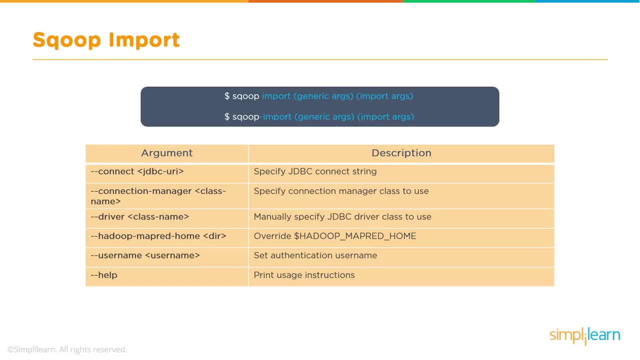 Username, set authentication username and, of course, help print uses instructions And with the export you'll see that we can specify the JDBC connect string. specify the ConnectionManager class to use manually. specify JDBC driver class to use. You do have to let it know to override the Hadoop MapReduceHome. 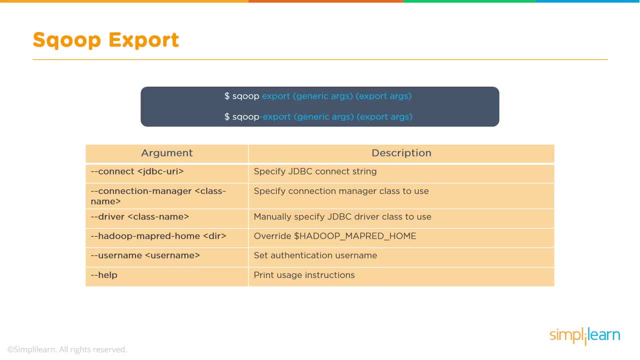 and that's true on both of these- And set authentication username and finally, you can print out all your help setup. So you can see the format for Scoop is pretty straightforward, both import and export. So let's continue on our path and look at Scoop processing. 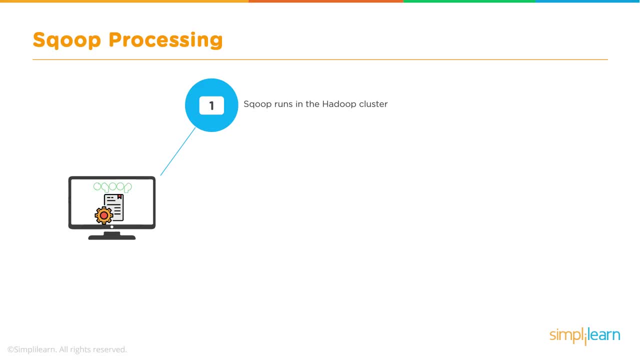 and what the computer goes through for that. And when we talk about Scoop processing, first Scoop runs in the Hadoop cluster. It imports data from the RDBX, The NoSQL database, to the Hadoop file system. So remember it might not be importing the data from a RDBMS. 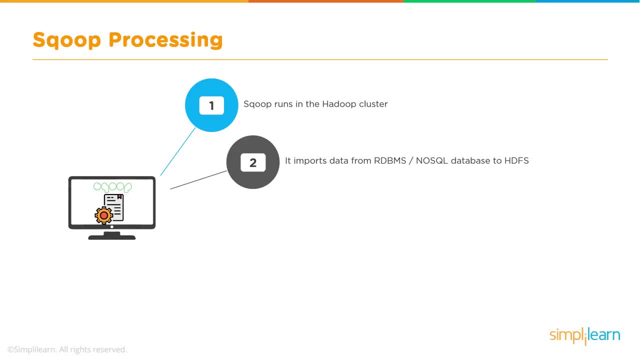 it might actually be coming from a NoSQL, and there's many out there. It uses mappers to slice the incoming data into multiple formats and load the data into HDFS. It exports data back into an RDBMS, while making sure that the schema of the data in the database is maintained. 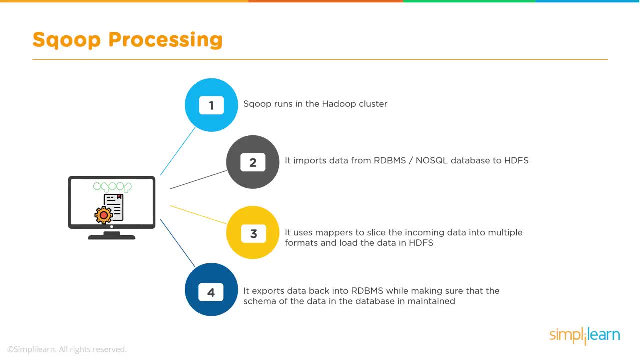 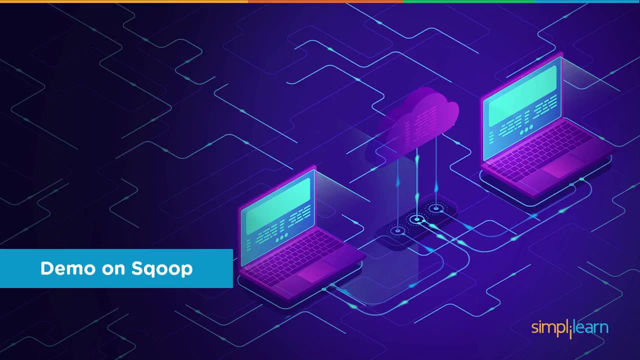 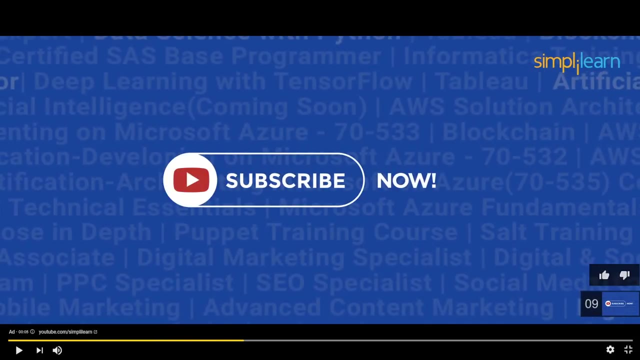 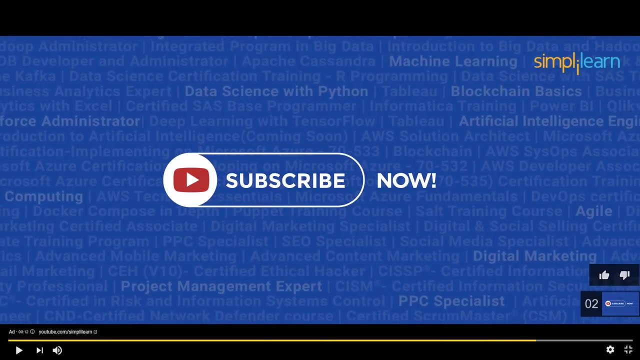 So now that we've looked at the basic commands in our Scoop, in the Scoop processing, at least the basics as far as theory is concerned- let's just jump in and take a look at a demo on Scoop. For this demo, I'm going to use our Cloudera Quick Start. 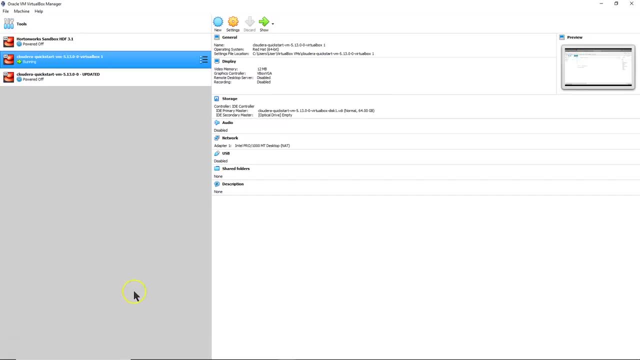 If you've been watching our other demos we've done, you'll see that we've been using that pretty consistently. Certainly this will work in any of your Horton Sandbox, which is also a single node testing machine. Cloudera is one of them. 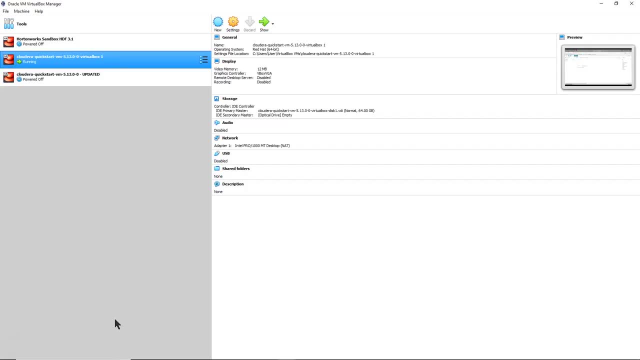 There's a Docker version instead of VirtualBox, And you can also set up your own Hadoop cluster Plan a little extra time. If you're not an admin, it's actually a pretty significant endeavor For an admin if you've been adminning Linux machines for a very long time. 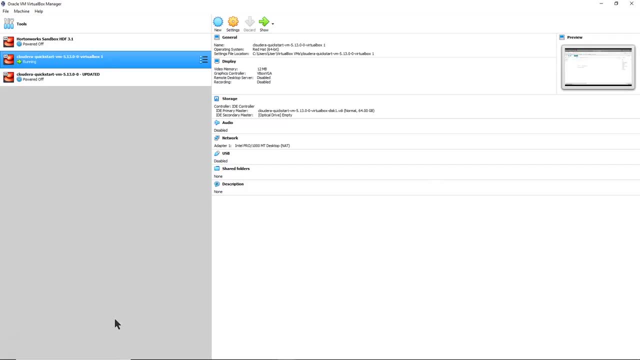 and you know a lot of the commands. I find, for most admins, it takes them about two to four hours the first time, Whereas the first time they go in and create a virtual machine and set up their own Hadoop. In this case, though, 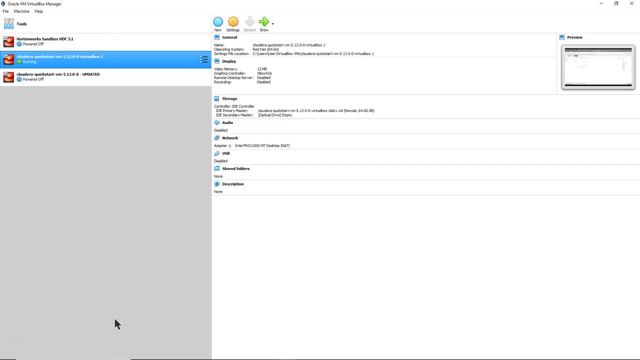 when you're just learning and getting set up, best to start with Cloudera. Cloudera also includes an installed version of MySQL. That way you don't have to reinstall the SQL version for importing data from and to Once you're in the Cloudera Quick Start. 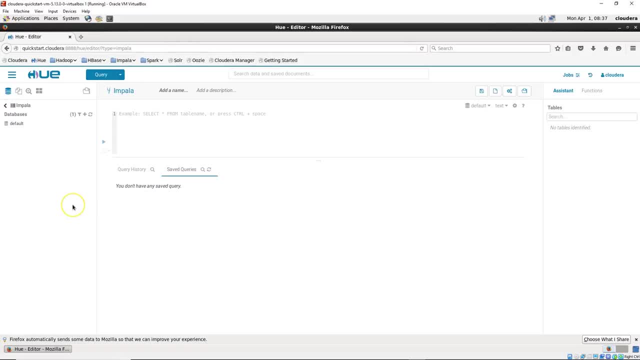 you'll see it opens a nice CentOS Linux interface And it has the desktop set up on there. This is really nice for learning. so you're not just looking at command lines And from in here it should open up a little bit and open up by default to Hue. 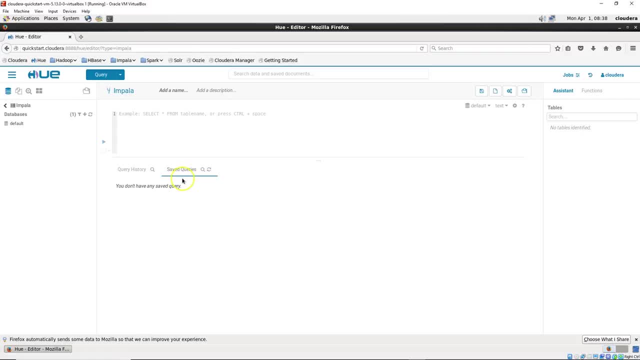 If not, you can click on Hue, Hue's kind of a fun little web-based interface. Under Hue I can go under Query, I can pick an editor And we'll go right down to Scoop. So now I'm just going to load the Scoop editor in our Hue. 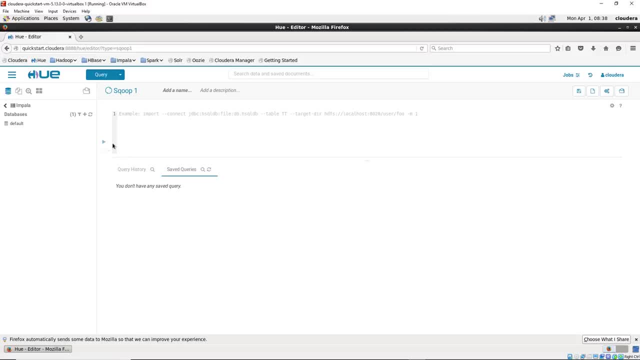 Now I'm going to switch over and do this all in command line. I just want to show that you can actually do this in Hue through the web-based interface. The reason I like to do the command line is specifically on my computer. it runs much quicker. 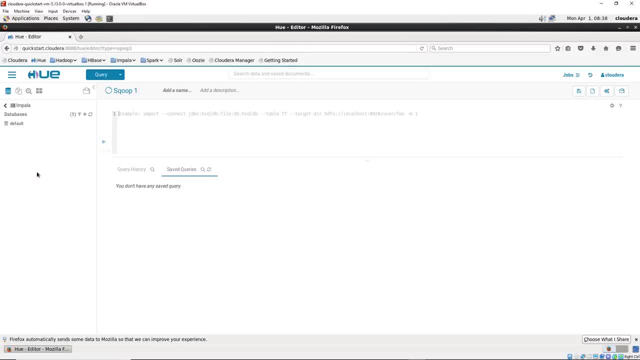 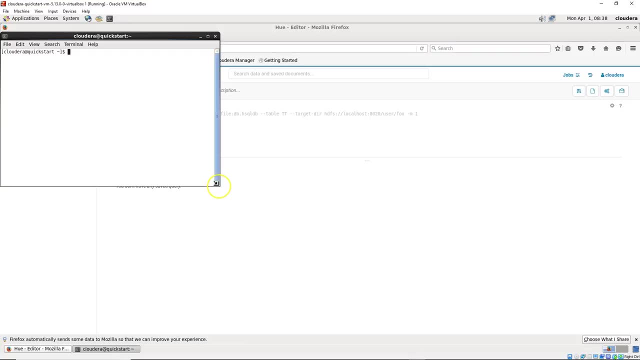 If I do the command line here and I run it, it tends to have an extra lag or an added layer in it. So for this we're going to go ahead and open our command line. The second reason I do this is we're going to need to go ahead and edit our MySQL. 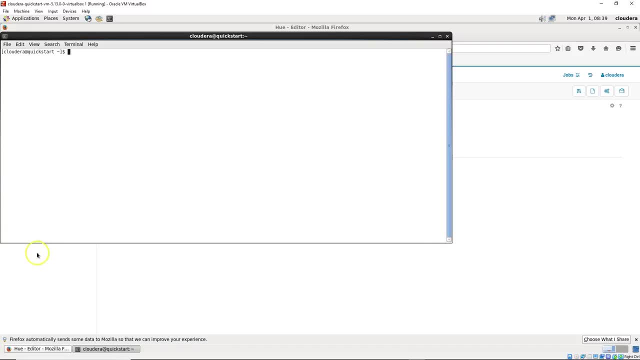 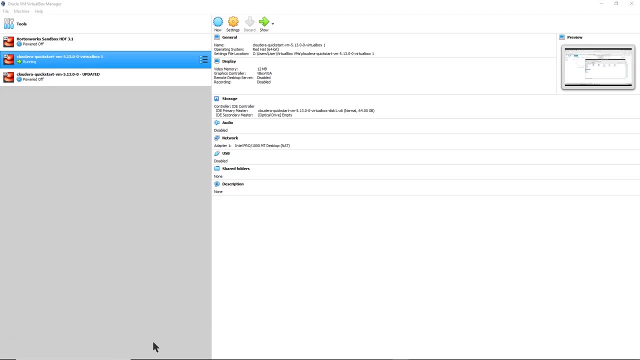 so we have something to scoop in. Otherwise I don't have anything going in there And of course we zoom in. We'll zoom in this and increase the size of our screen. So for this demo, our hands-on, I'm going to use Oracle VirtualBox Manager. 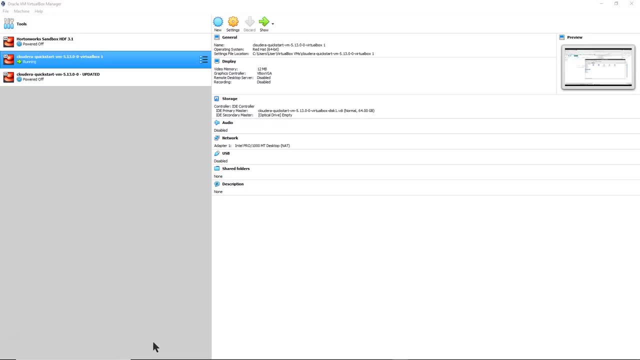 and the Cloudera Quick Start. If you're not familiar with this, we do have another tutorial we put out And you can send a note in the YouTube video below and let our team know and they'll send you a link. Or come visit wwwsimplylearncom. 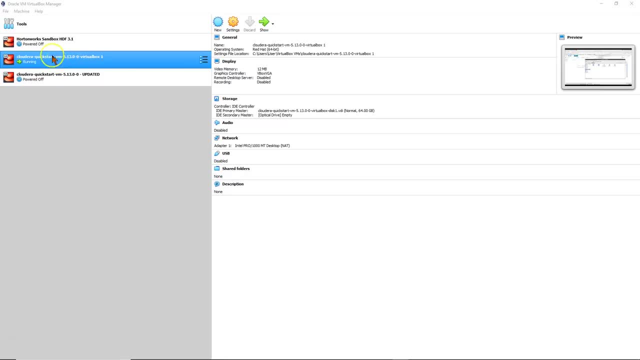 Now this creates a Linux box on my Windows computer, So we're going to be in Linux And it'll be the Cloudera version with Scoop. It will also be using MySQL MySQL Server Once inside the Cloudera VirtualBox. 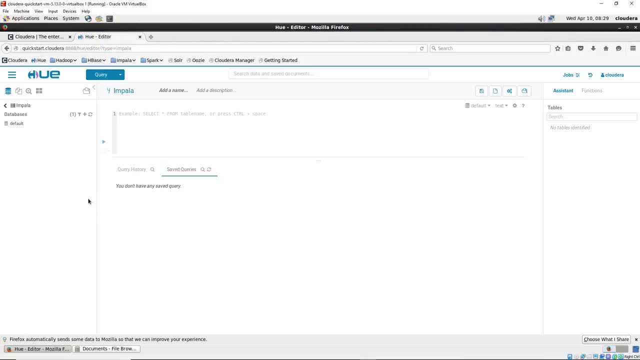 we'll go under the Hue Editor. Now we're going to do everything in Terminal Window, but I just want you to be aware that under the Hue Editor you can go under Query Editor and you'll see as we come down here. 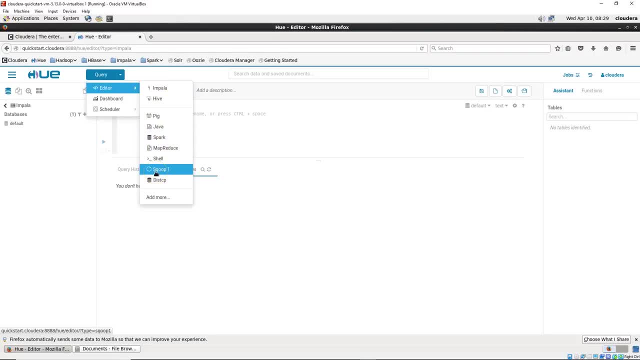 here's our Scoop on this, So you can run your Scoop from in here. Now, before we do this, we have to do a little exploration in MySQL or MySQL Server. That way we know what data is coming in. So let me go ahead and open up a Terminal Window. 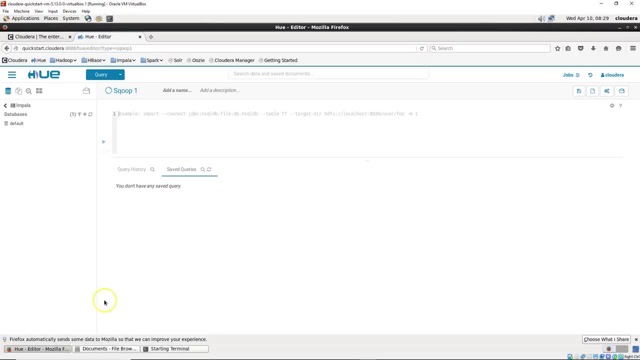 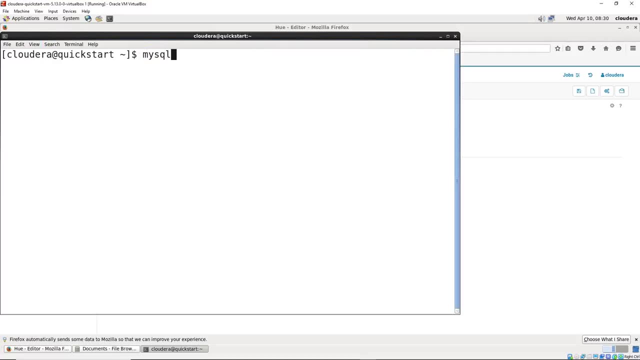 In Cloudera. you have a Terminal Window at the top here that you can just click on and open it up. And let me just go ahead and zoom in on here. Go View and Zoom In. Now to get into MySQL Server, you simply type in MySQL. 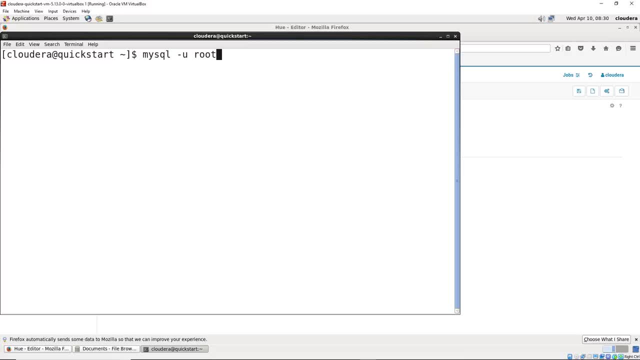 And this part will depend on your setup. Now the Cloudera Quick Start comes up that the username is Root and the password is Cloudera. Kind of a strange quirk is that you can put a space between the minus U and the root. 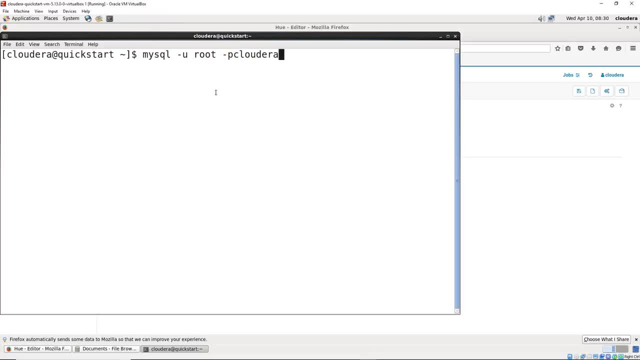 but not between the minus P and the Cloudera. Usually you'd put in a minus capital P and then it prompts you for your password on here For this demo. I don't worry too much about you knowing the password on that, so we'll just go right into MySQL Server. 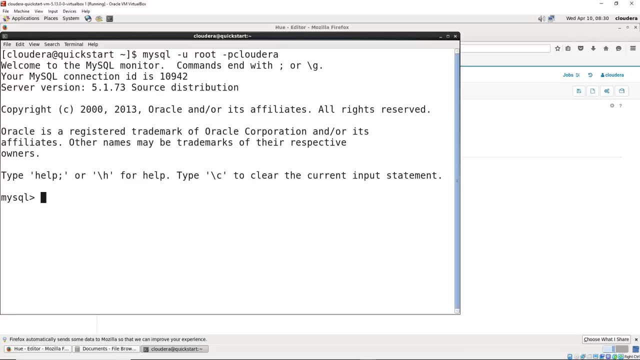 since this is the standard password for this Quick Start And you can see we're now into MySQL And we're going to do just a couple of quick commands. in here There's Show Databases and you follow by the semicolon. That's standard in most of these shell commands. 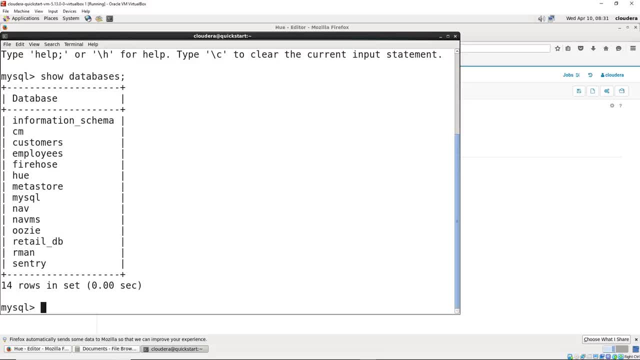 so it knows it's the end of your shell command And you'll see in here in the Quick Start, Cloudera, Quick Start. the MySQL comes with a standard set of databases. These are just some of these have to do with the Uzi. 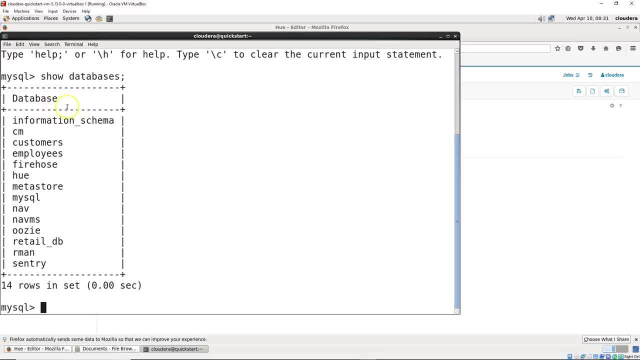 which is the Uzi part of Hadoop, where others of these like Customers and Employees and stuff like that. those are just for demo purposes. They come as a standard setup in there so that people going in for the first time have a database to play with. 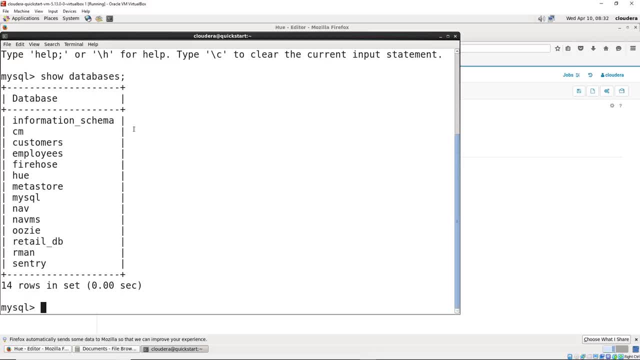 which is really good for us. so we don't have to recreate those databases And you will see on the list here we have a Retail underscore DB And then we can simply do Use Retail underscore DB. This will set that as a default in MySQL. 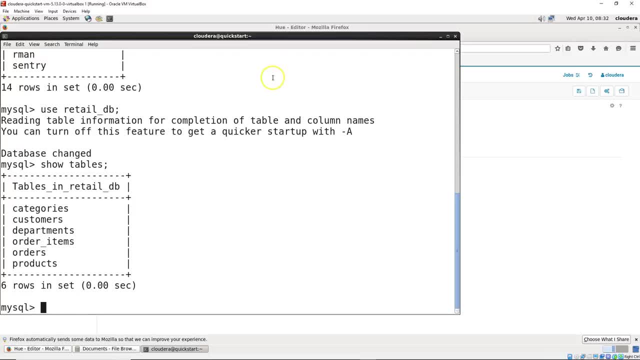 And then we want to go ahead and show the tables. And if we show the tables you can see under the database, the Retail DB database, we have Categories, Customers, Departments, Order Items, Orders, Products. So there's a number of tables in here. 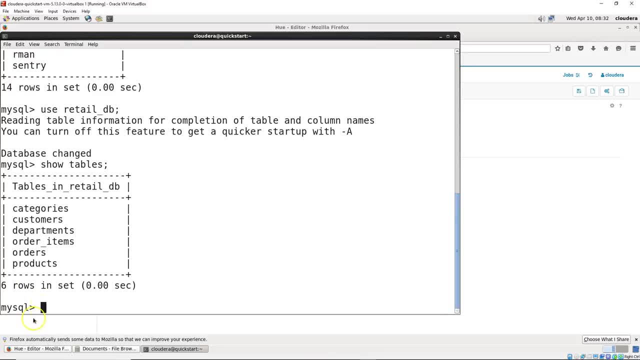 And we're going to go ahead and just use a standard SQL command. And if you did our Hive language, you'll note, remember it's the same for HQL. also on this, We're just going to select star everything from Departments. So there's our Departments table. 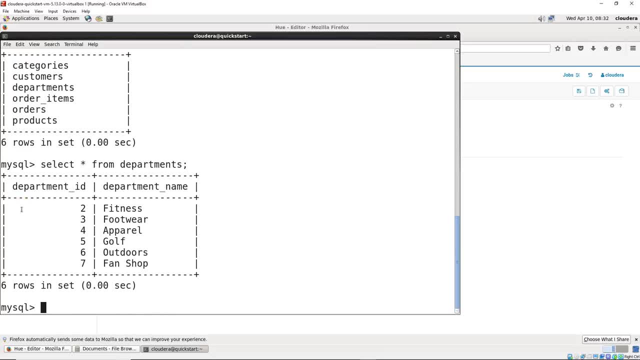 And we're going to list everything on the Departments table And you'll see we have six lines in here and it has a Department ID and a Department Name: Two for Fitness, two for Footwear, so on and so forth. Now, at this point, 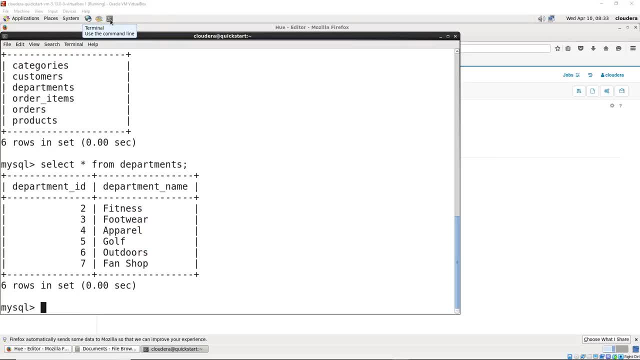 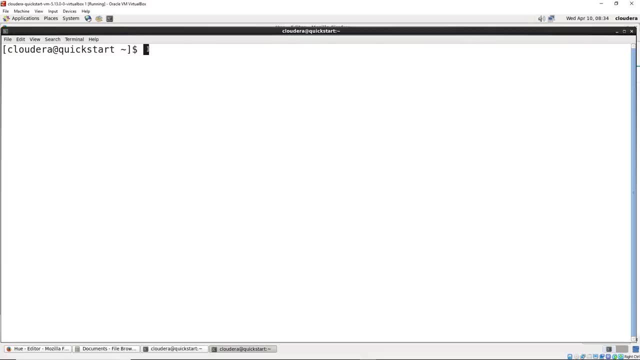 I can just go ahead and exit, But it's kind of nice to have this data up here so we can look at it and flip back and forth between the screens. So I'm going to open up another Terminal window And we'll go ahead and zoom in on this also. 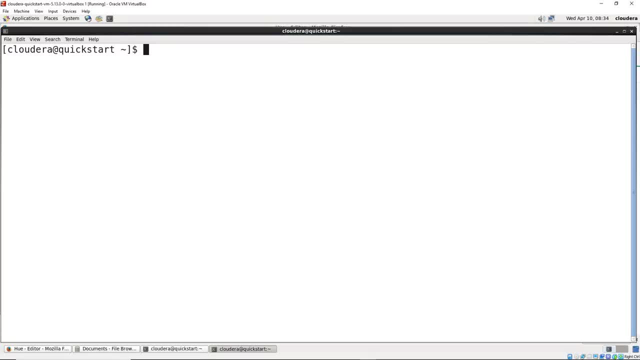 And it isn't too important for this particular setup, but it's always kind of fun to know what setup you're working with, What is your hostname, And so we'll go ahead and just type that in. This is a Linux command and it's. 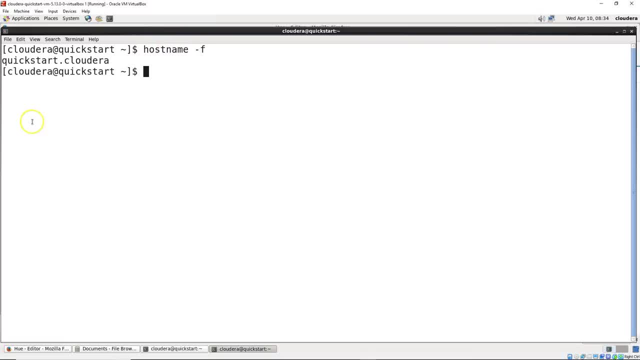 hostname minus f, We're on Quickstart Cloudera. No surprise there. Now this next command is going to be a little bit longer, because we're going to be doing our first scoop command And I'm going to do two of them. 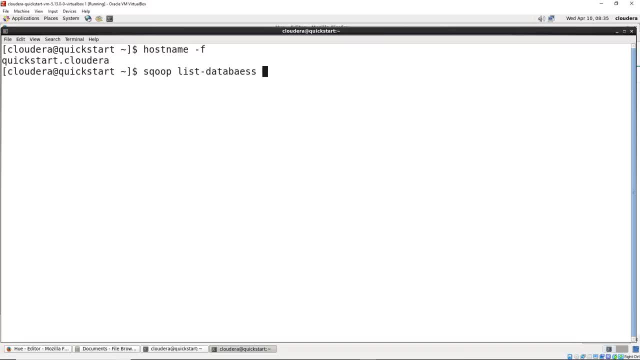 We're going to list databases and list tables. This is going to take just a moment to get through this because there's a bunch of stuff going on here. So we have scoop, we have list databases, we have connect And under the connect command, 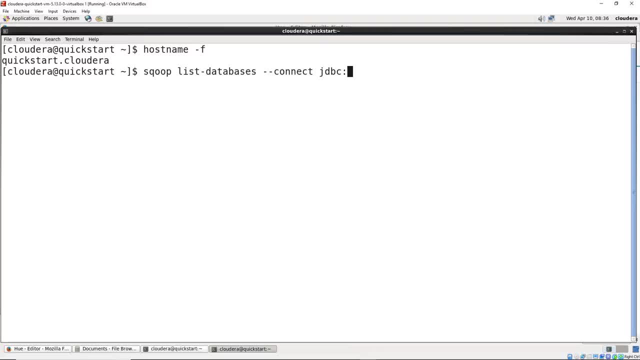 we need to let it know how we're connecting. We're going to use the JDBC MySQL, So you'll see that if you're doing an SQL database, that's how you start it off with. And then the next part. this is where you have to go look it up. 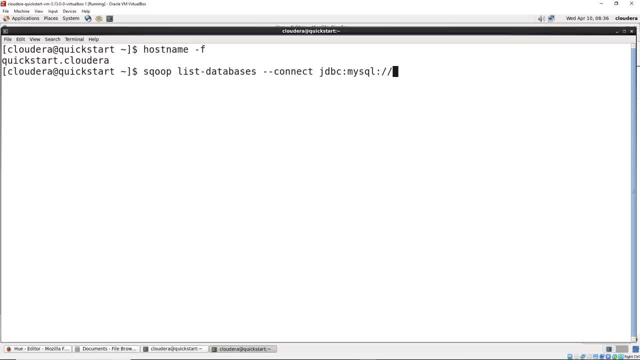 It's however it was created. So if your admin created a MySQL server with a certain setup, that's what you have to go by And you'll see that usually they list this as localhost, So you'll see something like localhost. sometimes There's a lot of different formats. 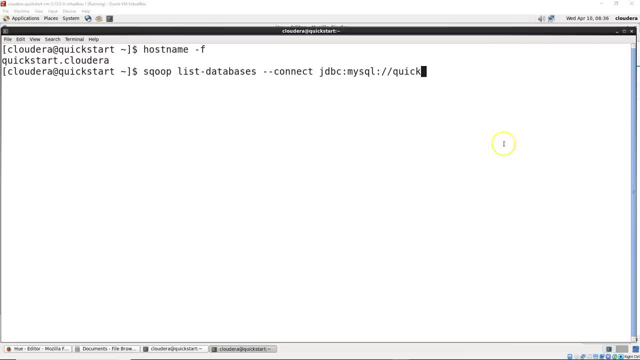 But the most common is either localhost or the actual connection. So in this case we want to go ahead and do port 3306.. And so quickstart is the name of the localhost database and how it's hosted on here And when you set up the quickstart. 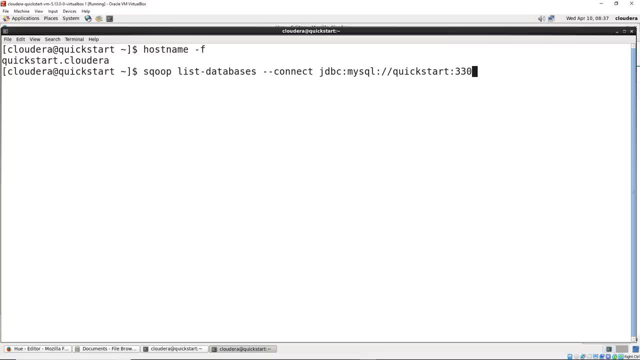 for Hadoop under Cloudera. it's port 3306 is where that's coming in, So that's where all that's coming from, And so there's our path for that. And then we have to put in our password. We type in the type: password. 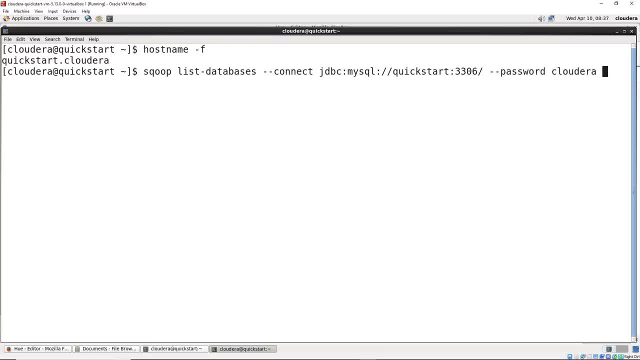 If you look it up, password on the Cloudera, quickstart is Cloudera And we have to also let it know the username. And again, if you're doing this minus capital, you can actually just do it for a prompt for the password. 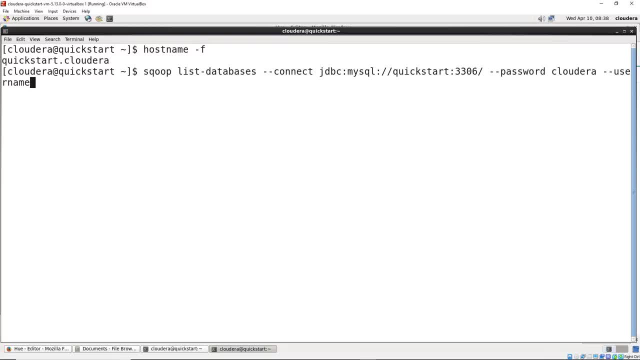 So if you leave that out, it'll prompt you, But for this it doesn't really matter. I don't care. if you see my password, It's the default one for Cloudera quickstart, And then the username on here is simply root. 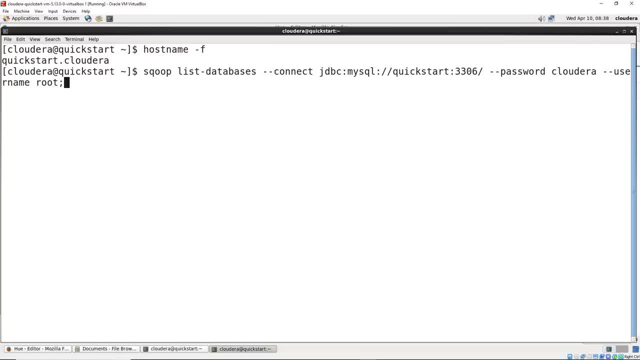 And then we're going to put our semicolon at the end And so we have here our full setup. Then we go ahead and list the databases And you'll see you might get some warnings on here. I haven't run the updates on the quickstart. 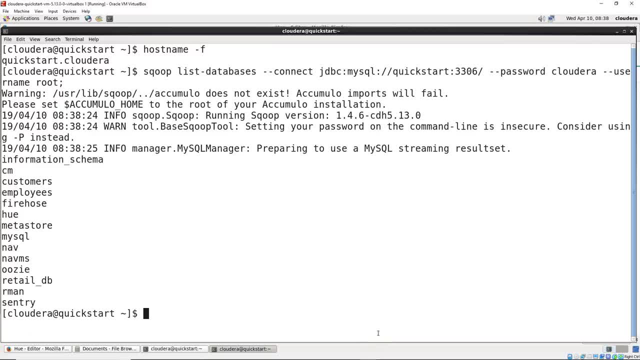 I suggest you're not running the updates either. if you're doing this for the first time, just do some reformatting on there And it quickly pops up and you can see. here's all of the tables we went in there And if we go back to 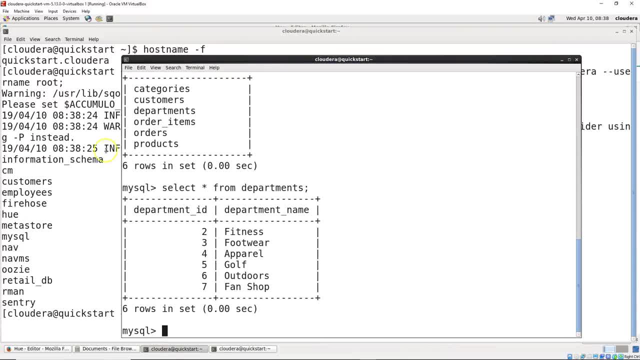 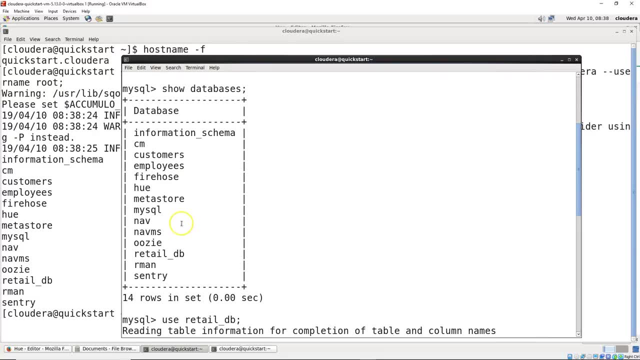 on the previous window. we should see that these tables match. So here we come in and here we have our databases And you can see back up here we had the CM customers, employees and so on. So the databases match. And then we want to go ahead and list the 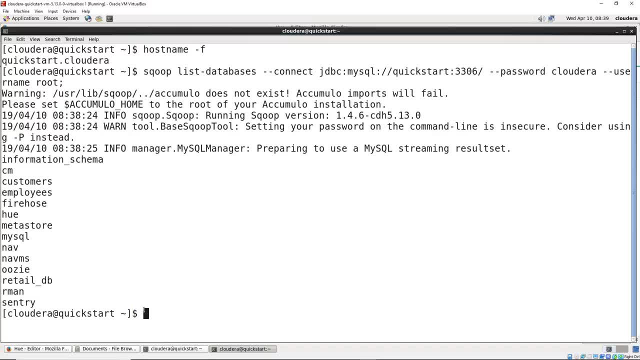 tables for a specific database, So let's go ahead and do that. I'm a very lazy typist And you can see here: scoop list databases. We're just going to go back and change this from databases to list tables, So we want to list the tables in here. 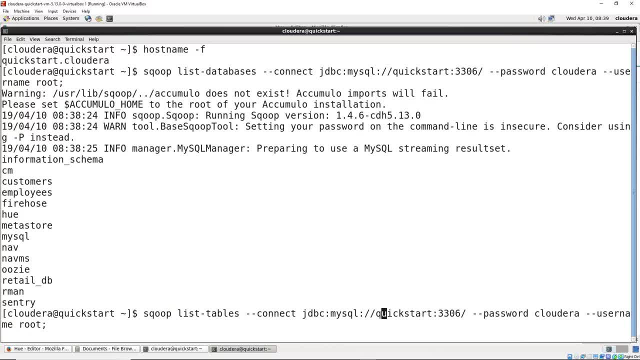 Same connection. So most of the connection is the same, except we need to know which tables we're listing. An interesting fact is you can create a table without being under a database, So if you left this blank, it will show the open tables that aren't connected directly to a database. 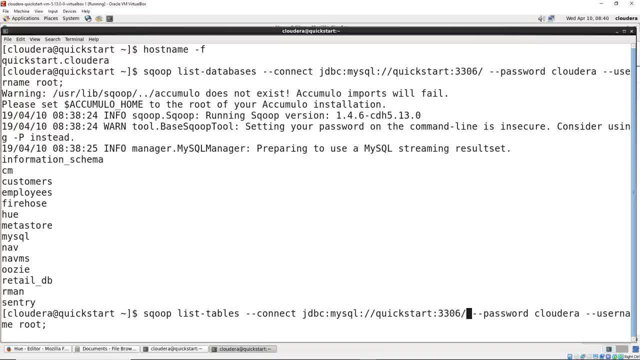 or under a database. But what we want to do is, right past this last slash on the 3306, we want to put that underscore DB, Because that's the database we're going to be working with And this will go in there and show the tables. 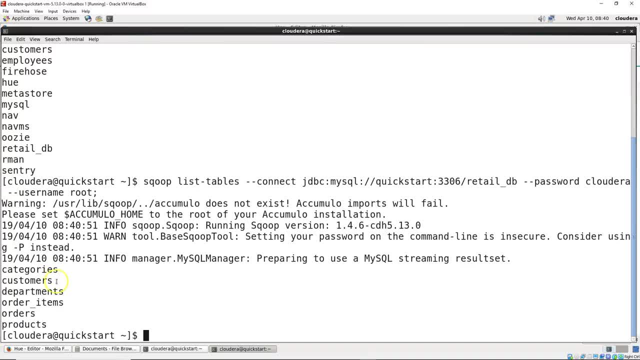 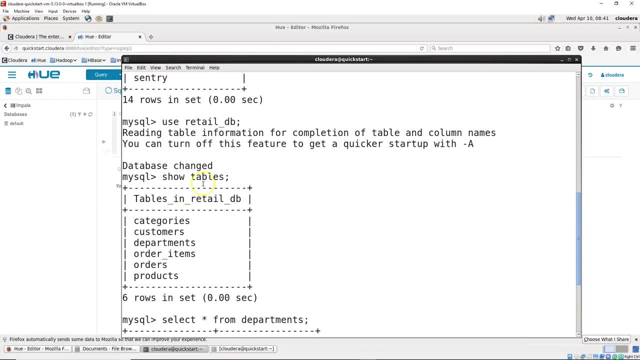 listed under that database. And here we go, We've got categories, customers, departments, order items and products. If we flip back here real quick, there it is the same thing we had. We had categories, customers, departments. 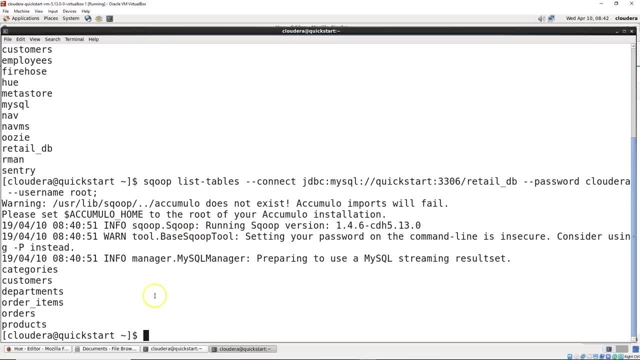 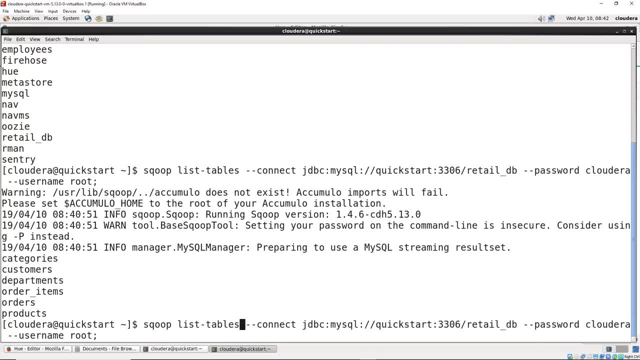 order items and so on, And so let's go ahead and run our first import command. And again, I'm that lazy typer. So we're going to do scoop And instead of list tables, we want to go ahead and import. 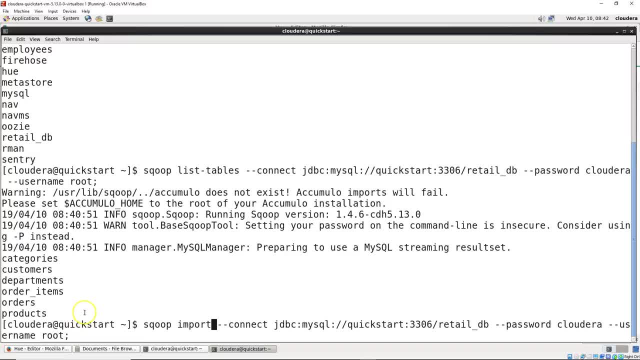 So there's our import command, And so once we have our import command in there, then we need to tell it exactly what we're going to import. So everything else is the same. We're importing from the retail DB, so we keep that. 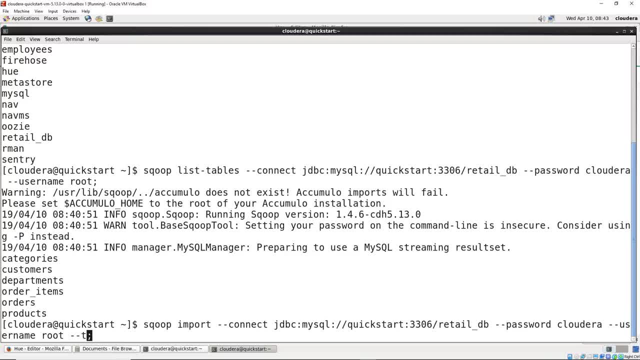 And then at the very end we're going to tag on dash dash table That tells it, so we can tell it what table we're importing from And we're going to import departments There we go. So this is pretty straightforward, because what's nice about this is 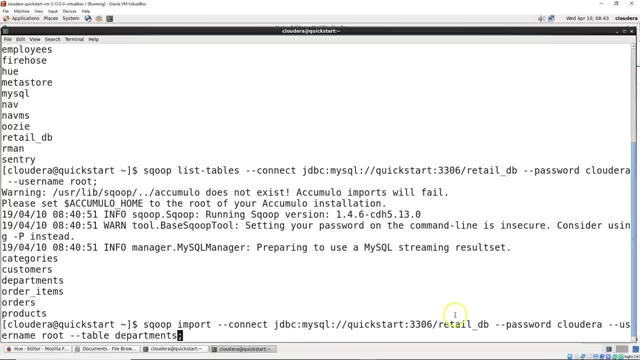 you can see, the commands are the same. I've got the same connection. I change it for whatever database I'm in. Then I come in here. Our password and the username are going to be the same. That's all under the MySQL server setup, And then we let it know what table. 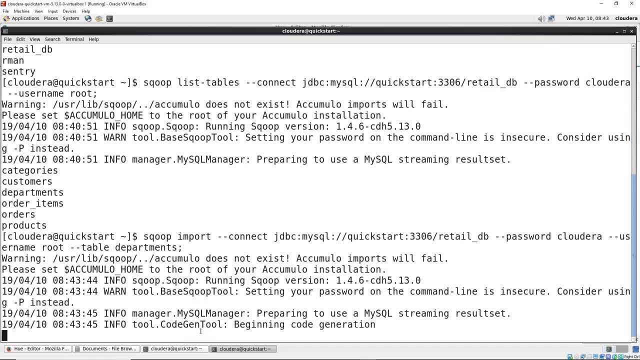 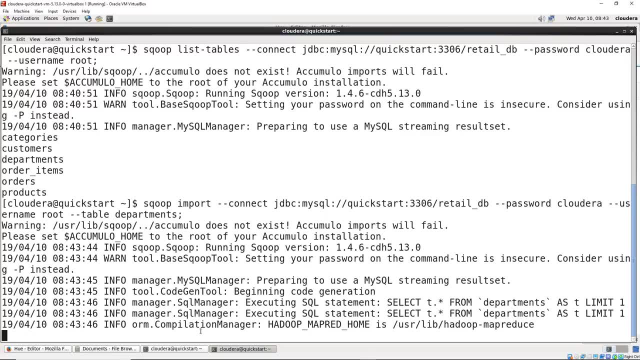 we're entering in, We run this And this is going to actually go through the mapper process in Hadoop. So this is a mapping process. It takes the data and it maps it up to different parts in the setup in Hadoop on there. 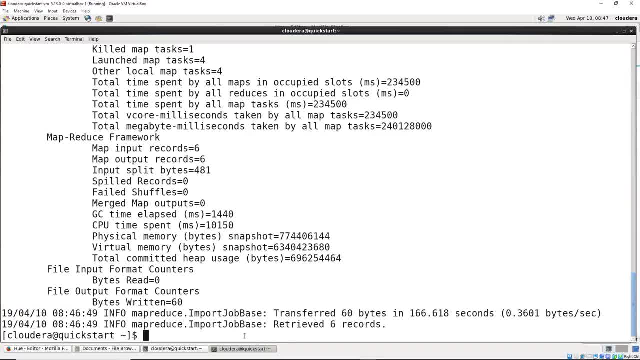 and then saves that data into the Hadoop file system, And it does take it a moment to zip through, which I kind of skipped over for you, Since it is running a. you know it's designed to run across a cluster, not on a single node. 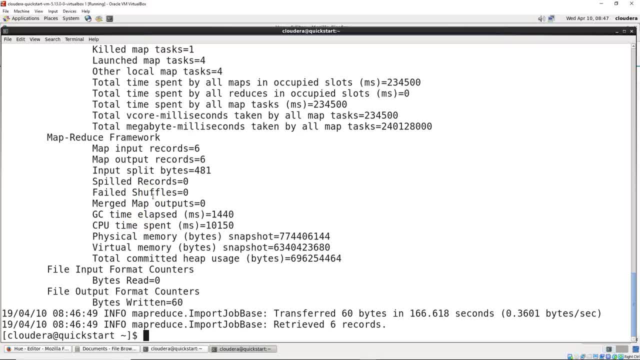 So when you're running it on a single node, it's going to run slow, even if you dedicate a couple cores to it. I think I put dedicated four cores to this one, And so you can see right down here we get to the end. It's now mapped. 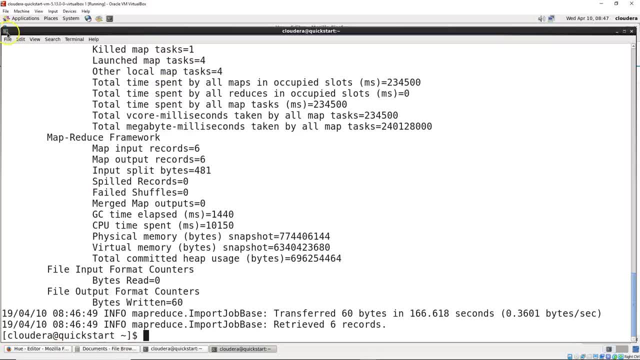 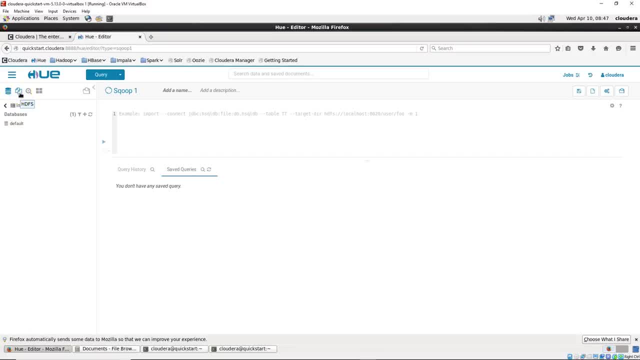 in that information And then we can go in here, We can go under, we can flip back to our Hue And under Hue on the top I have there's databases and the second icon over is your Hadoop file system. 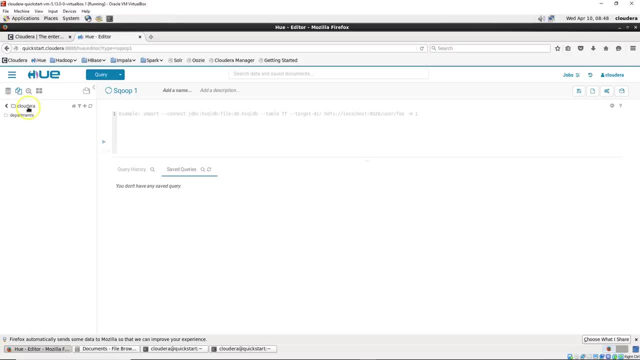 And we can go in here and look at the Hadoop file system And you'll see it show up underneath our documents. There it is departments, Cloudera departments, And you can see there's always a delay when I'm working in Hue, which I don't like. 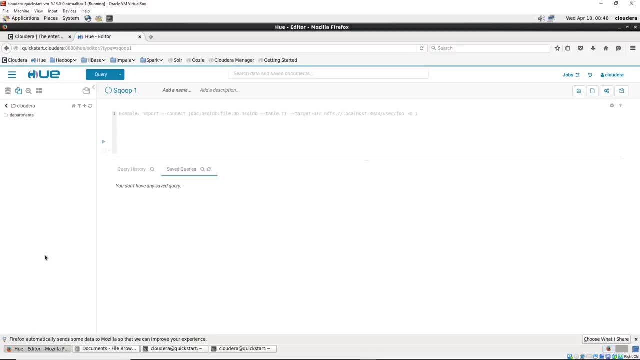 And that's the quick start issue. That's not necessarily running it on a server. When I'm running it on a server you pretty much have to run through some kind of server interface. I still prefer the terminal window. It still runs a lot quicker. 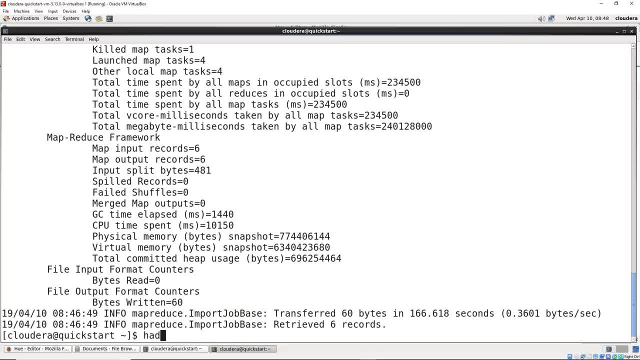 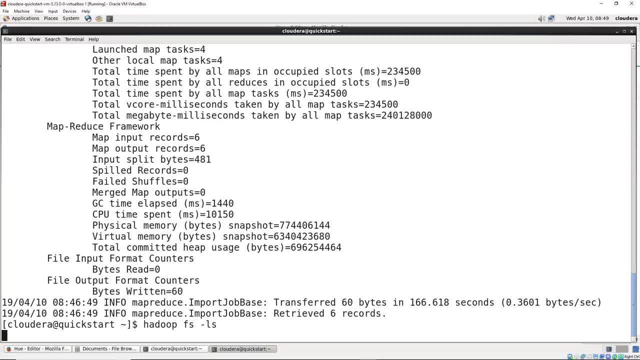 We'll flip back on over here to the command line And we can do the Hadoop type in the Hadoop fs and then list minus ls And if we run this you'll see underneath our Hadoop file system there is our departments. 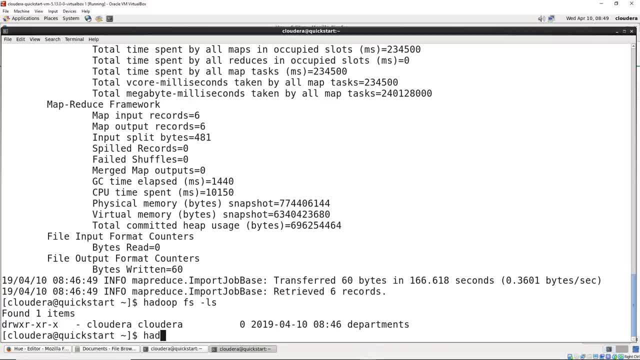 Which has been added in And we can also do Hadoop fs And this is kind of interesting For those who've gone through the Hadoop file system and everything. you'll recognize this on here. I'm going to list the contents of departments. 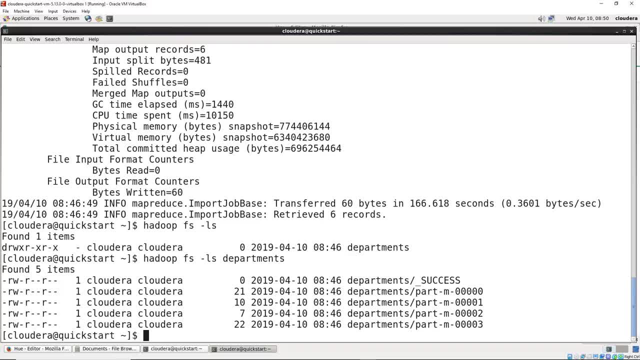 And you'll see, underneath departments we have part m: 000, 001,, 002, 003.. And so this is interesting, because this is how Hadoop saves these files. This is in the file system. This is not in Hive. 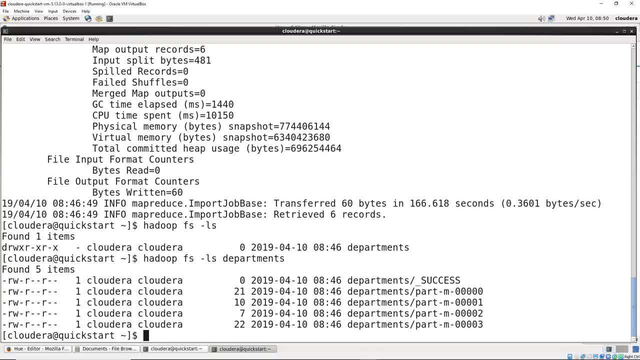 So we didn't directly import this into Hive. We put this in the Hadoop file system. Depending on what you're doing, you would then write the schema for Hive to look at the Hadoop file system. Certainly visit our Hive tutorial for more information. 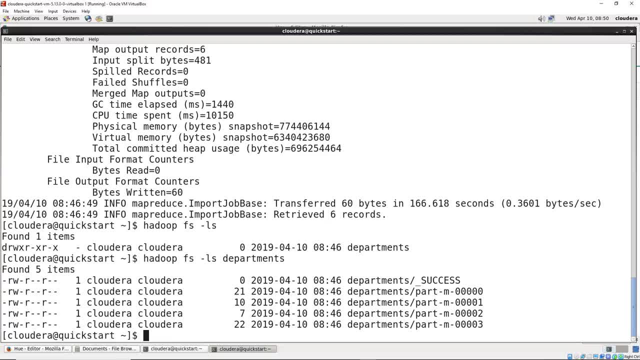 on Hive specific. So you can see in here are different files that it forms, that are part of departments, And we can do something like this. We can look at the contents of one of these files: fs minus ls, or a number of the files. 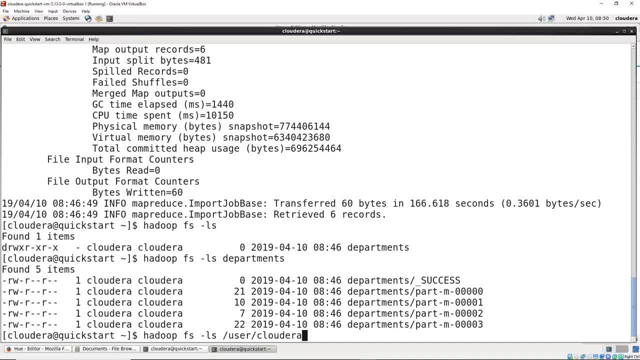 And we'll simply do the full path, which is user Cloudera, And then we already know. the next one is department, And then, after departments, we're going to put slash part star. So this is going to say anything that has part in it. 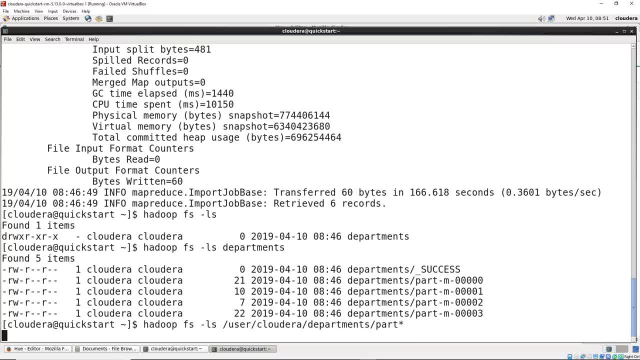 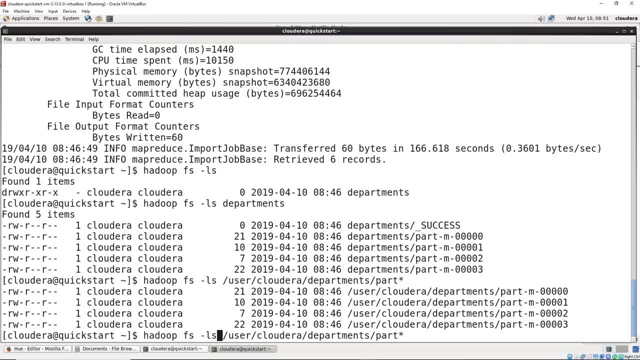 So we have part dash m 000 and so on. We can go ahead and cat Use that cat command or that list command to bring those up, And then we can use the cat command to actually display the contents, And that's a. 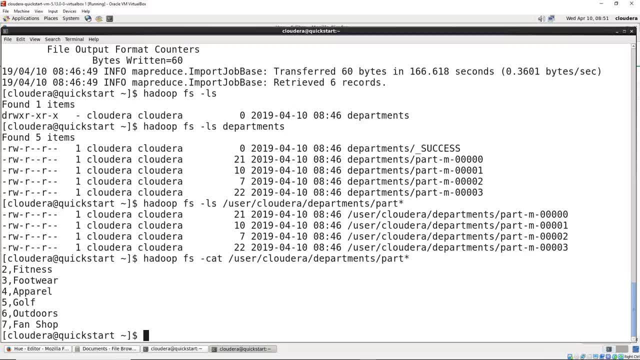 Linux command: Hadoop. Linux command to cat catinate, Not to be confused with catatonic catastrophic. There's a lot of cat got your tongue And we see here fitness footwear apparel That should look really familiar because that's what we had. 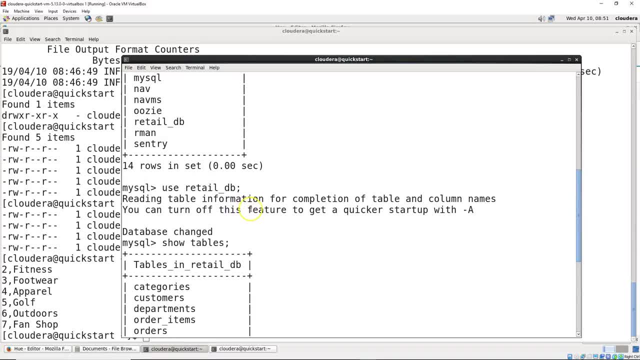 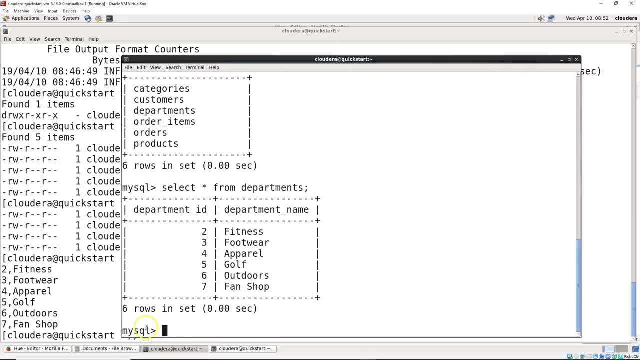 in our MySQL server. When we went in here we did a select all on here. There it is Fitness, footwear, apparel, golf, outdoors and fan shop, And then, of course, it's really important let's look back on over here to be able to. 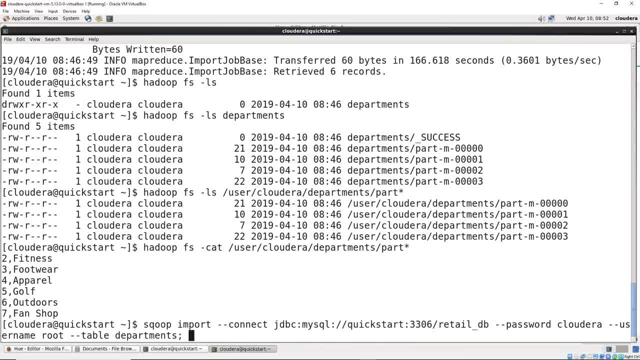 tell it where to put the data. So we go back to our import command. So here's our scoop: import: We have our connect, We have the db underneath our connection, our MySQL server. We have our password, our username, the table going. 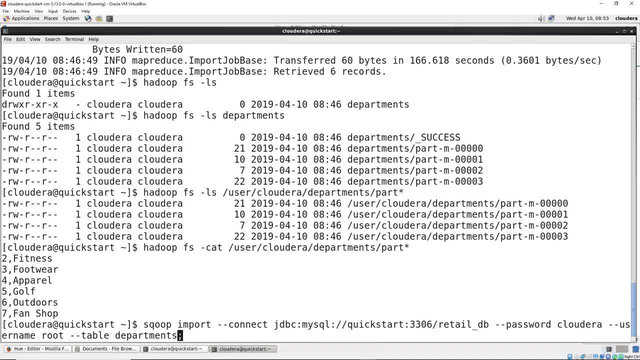 where it's going to, I mean the table, where it's coming from, And then we can add a target on here. We can put in target dash directory And you do have to put the full path. That's a Hadoop thing. It's a good practice. 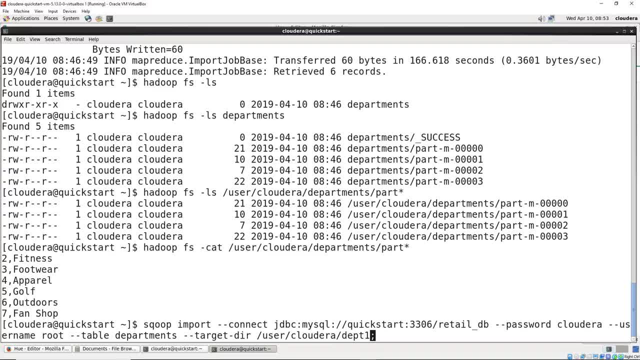 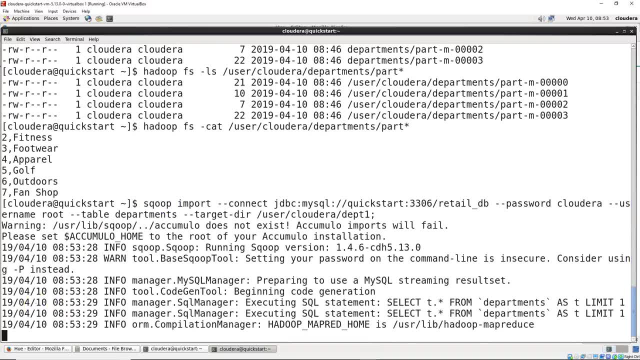 to be in And we're going to add it to department. we'll just do department one, And so here we now add a target directory in here and user cloud era department one. And this will take just a moment before, so I'll go ahead and skip over the process. 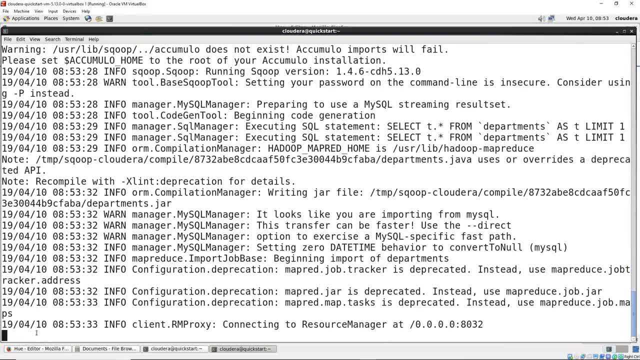 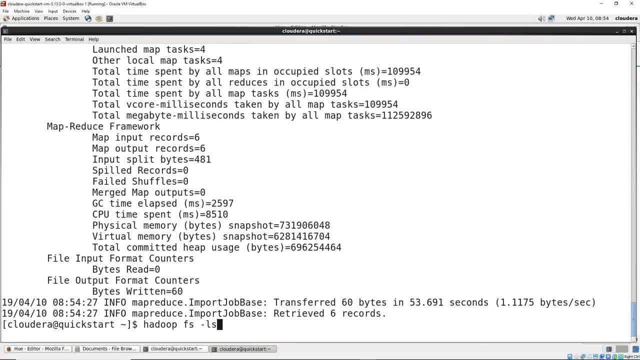 since it's going to run very slowly. It's only running on, like I said, a couple cores on a single node And now we can do the Hadoop. Let's just do the up arrow File system list. We want just straight list. 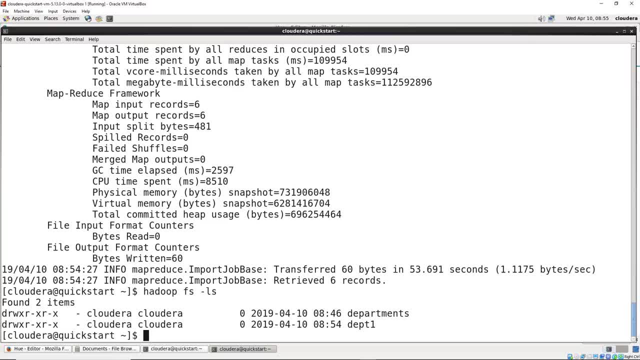 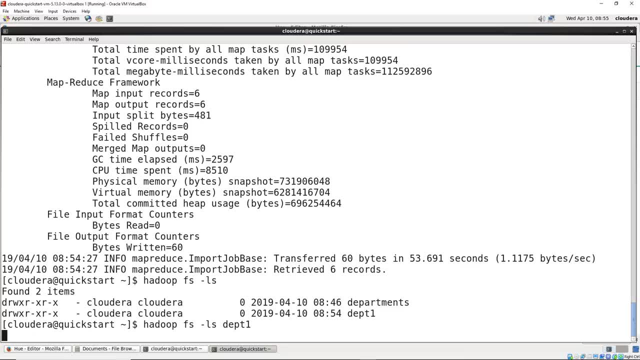 And when we do the Hadoop file system minus ls or list, you'll see that we now have department one And we can of course do list department one And you can see we have the files inside department one And they mirrored what we saw before with the same files. 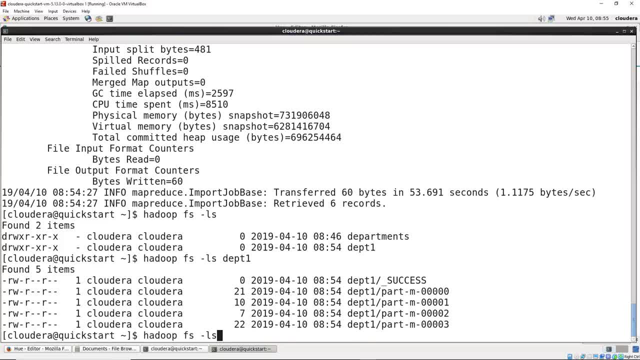 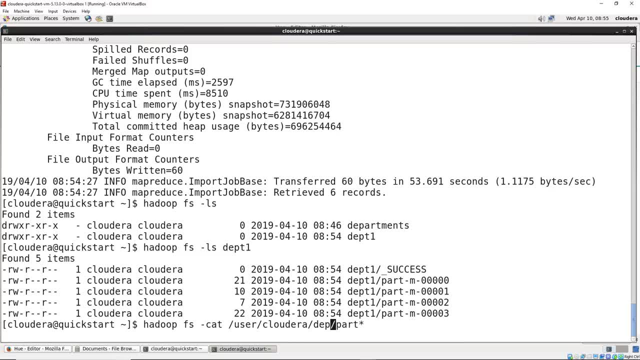 in there In the part mm 00 and so on. If we were to look at them, it would be the same thing we did before with the cat, except instead of departments we'd be department one. There we go, And then that's going to come up with the same data we had. 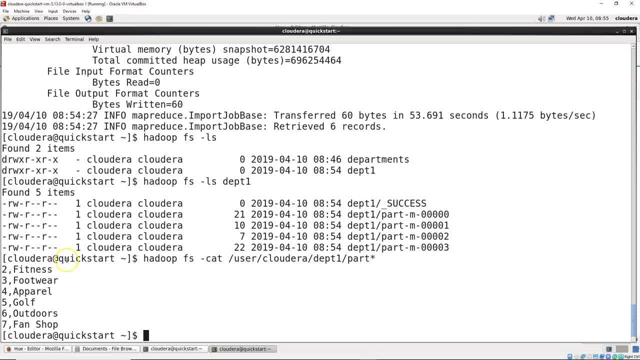 before Now. one of the important things when you're importing data- and it's always a question to ask- is: do you filter the data before it comes in? Do we want to filter this data as it comes in? so we're not storing? 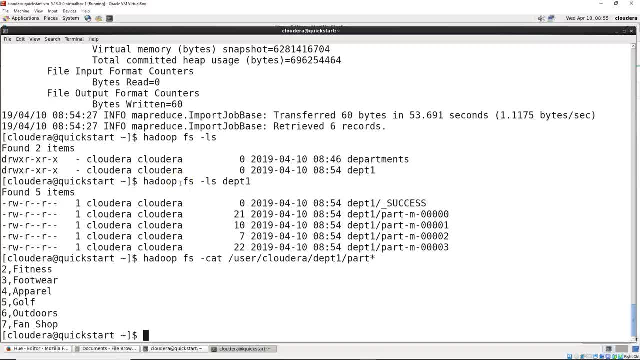 everything in our file system. You would think Hadoop big data, put it all in there. I know from experience that putting it all in there can turn a couple hundred terabytes into a petabyte very rapidly And suddenly you're having to really add on to. 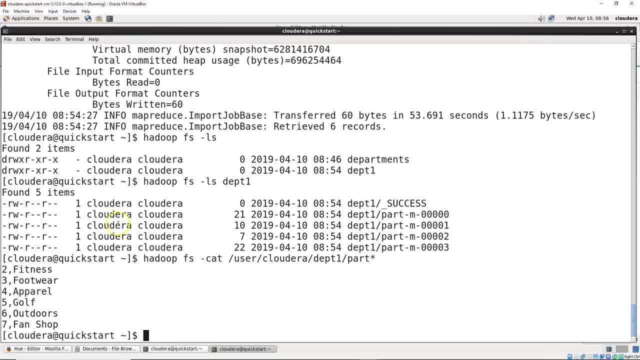 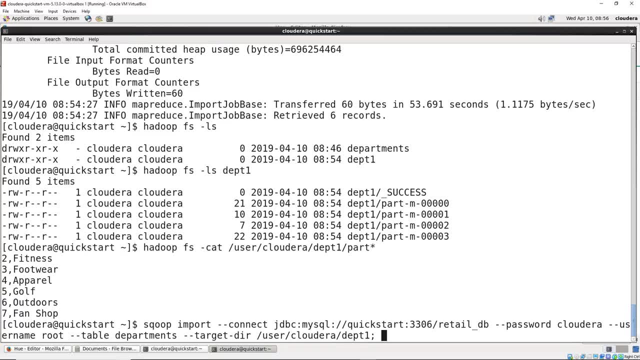 that data store and you're storing duplicate data sometimes, So you really need to be able to filter your data out, And so let's go ahead and use our up arrow to go to our last import, since it's still a lot the same stuff. 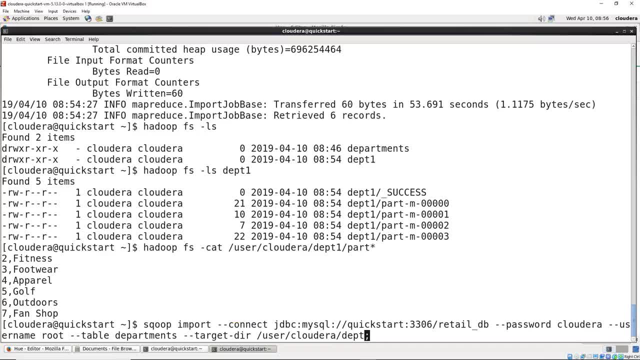 So we have all of our commands under import. We have the target. We're going to change this to department two, So we're going to create a new directory for this one. And then, after departments, there's another command that we didn't really. 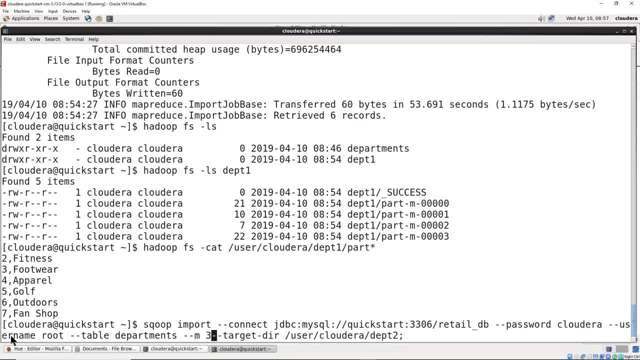 slide in here and that's our mapping, And I'll show you what this looks like in a minute. So we're going to put m3 in there. That doesn't have nothing to do with the filtering. I'll show you that in a second, though what that's for. 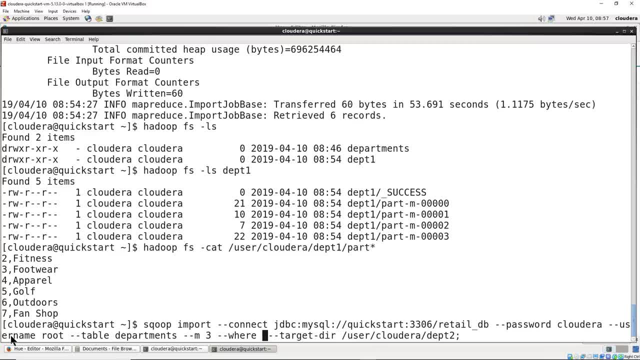 And we just want to put in where. So where and what is the where? In this case? we want to know where department id And if you want to know where that came from, we can flip back on over here. We have department underscore id. 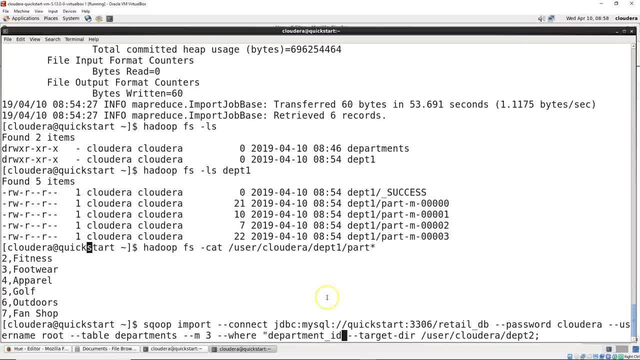 So this is where that's coming from. That's just the name of the column on here. So we come in here to department id is greater than four and a little logic there You can see where you'd use that for maybe creating buckets for ages you know, age from. 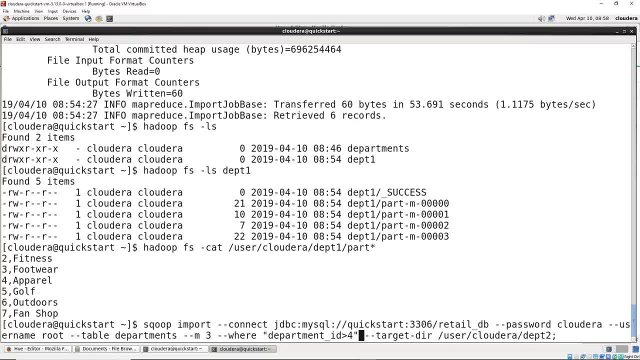 ten to fifteen, twenty to thirty You might be looking for. I mean, there's all kinds of reasons why you could use the where command on here And filter information out. Maybe you're doing word counting and you want to know words that are. 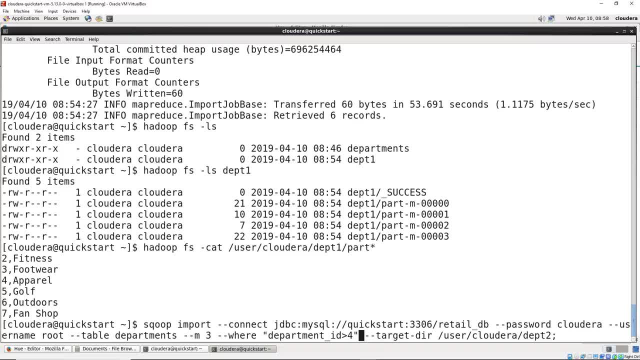 used less than a hundred times. You want to get rid of the and is, and and and a- all the stuff that's used over and over again. So we'll go ahead and put the where and then department id is greater than four, We'll go ahead and hit. 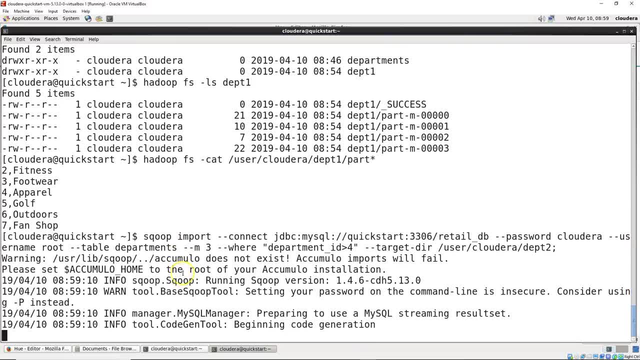 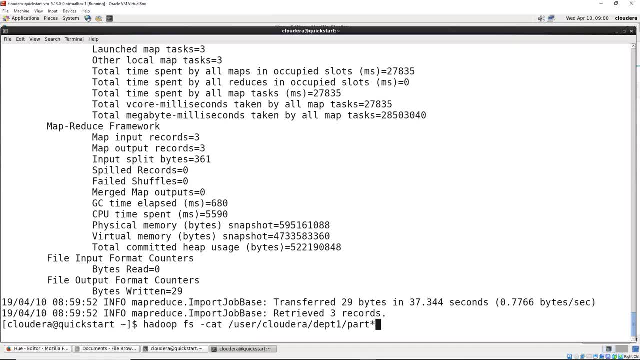 enter on here And this will create our department two set up on this And I'll go ahead and skip over some of the run time. Again, it runs really slow on a single node. Real quick page through our commands. Let's see, here we go. 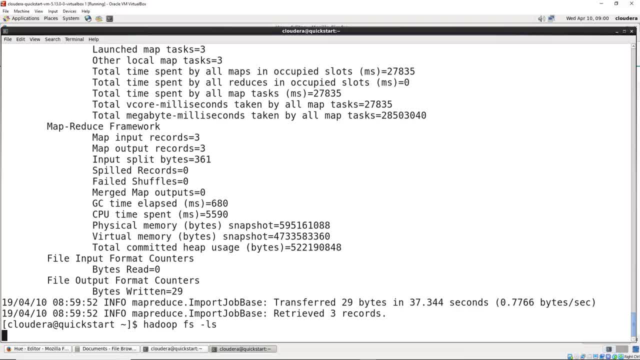 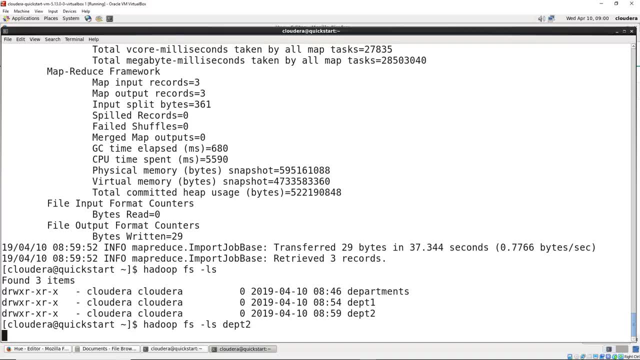 Our list And we should see underneath the list the department two on here now And there it is department two And then I can go ahead and do list department two. You'll see the contents in here And you'll see that there. 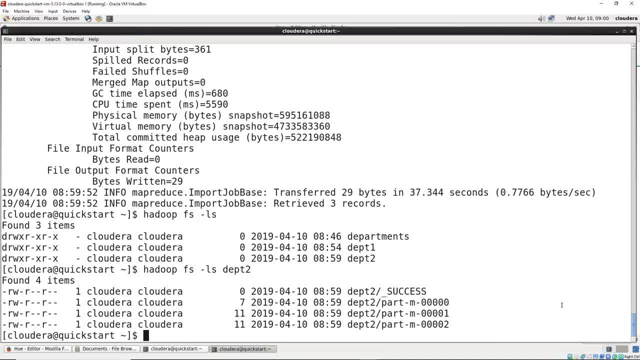 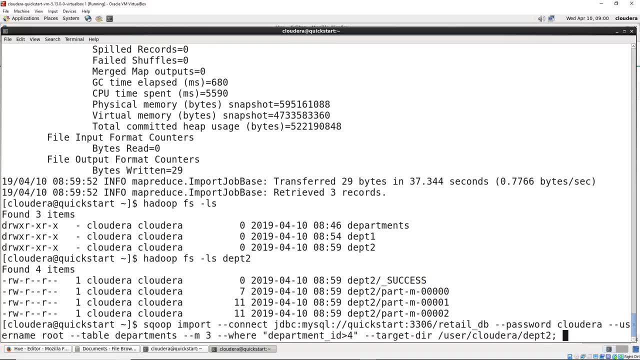 is only three maps And it could be that the data created three maps, But remember I set it up to only use three maps, So there's zero, one and two, And we can go ahead and do a cat on there. Remember this is. 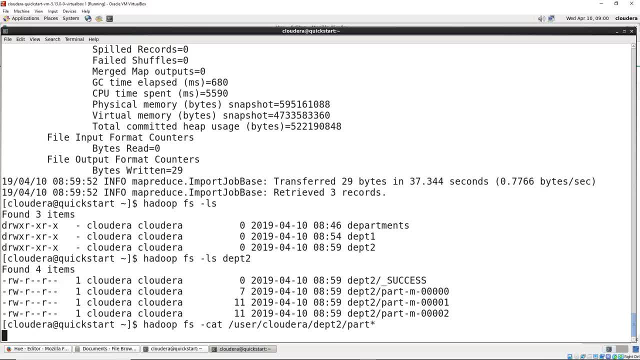 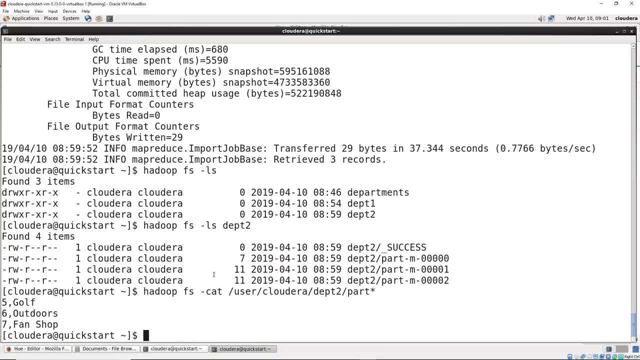 department two. So we want to look at all the contents of these three different files. And there it is, It's greater than four. So we have: golf is five, outdoor six, fan shop is seven. So we've effectively filtered out our data and just storing the data we want. 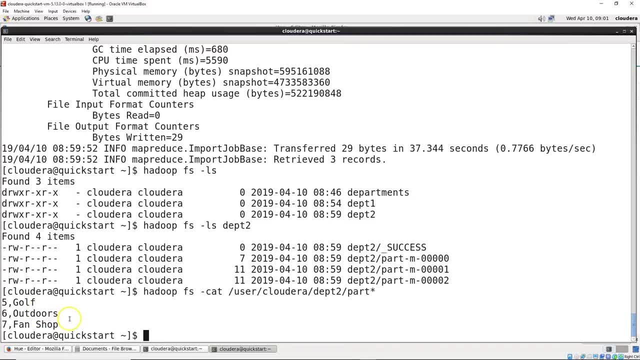 on our file system. So if you're going to store data on here, the next stage is to export the data. Remember, a lot of times you have MySQL Server and we're continually dumping that data into our long term storage and access the Hadoop file system. But what happens? 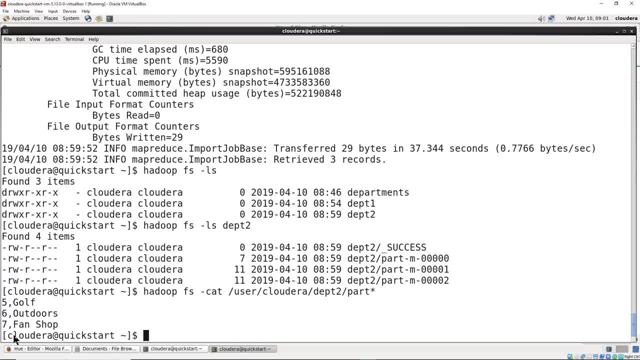 when you need to pull that data out and restore a database, Or maybe you have. you just merged with a new company- A favorite topic, merging companies and merging databases- That's listed under nightmare, and how many different names for company can you have? So 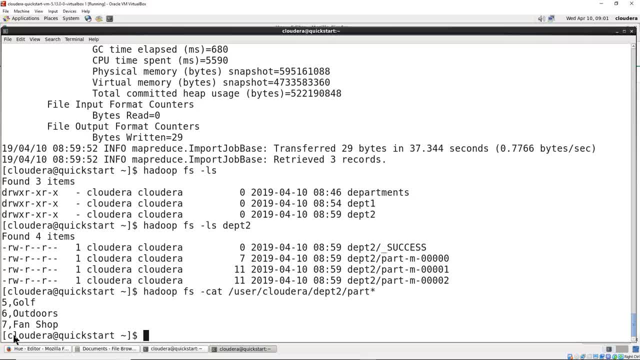 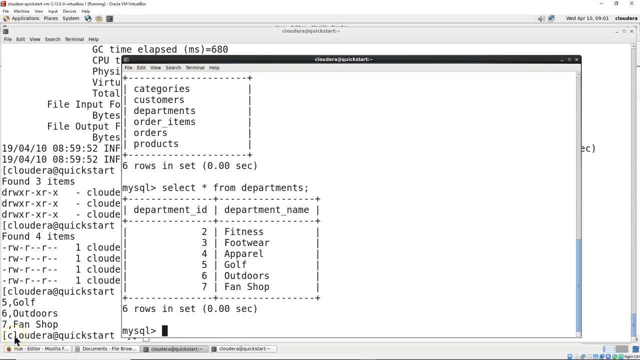 you can see where being able to export is also equally important, And let's go ahead and do that, And I'm going to flip back over to MySQL Server here And we'll need to go ahead and create our database we're going to export into. Now, I'm not 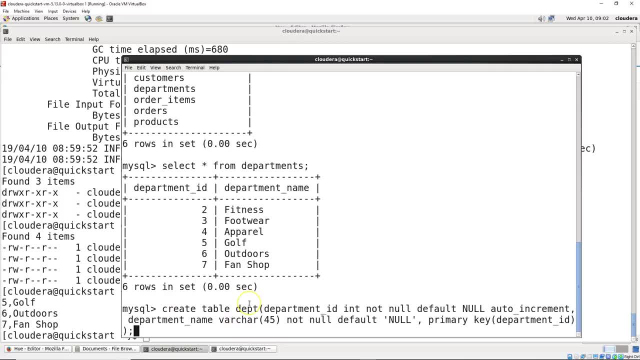 going to go too much in detail on this command. We're simply creating a table and the table's going to have. it's pretty much the same table we already have in here from departments, But in this case we're going to create a table called. 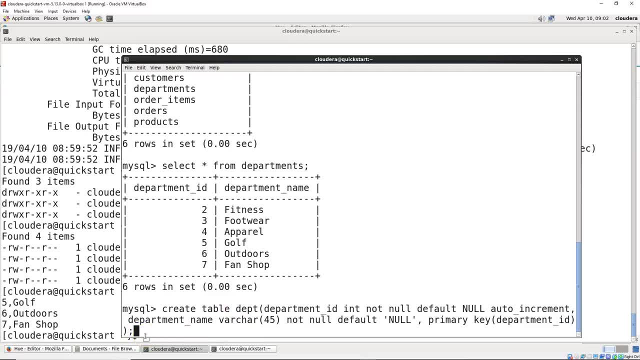 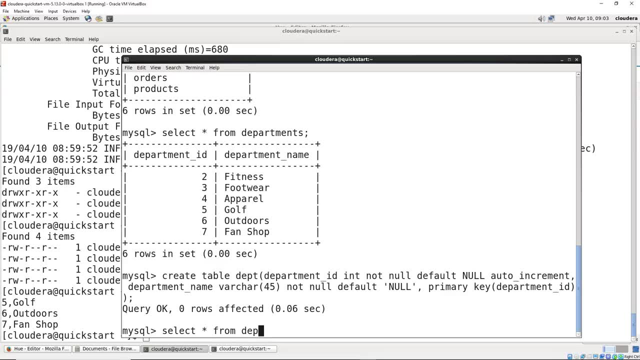 DEPT. So it's the same setup, but it's just going to. we're just giving it a different name, a different schema, And so we've done that and we'll go ahead and do a select star from DEPT. There we go, And it's empty. That's what we expect. 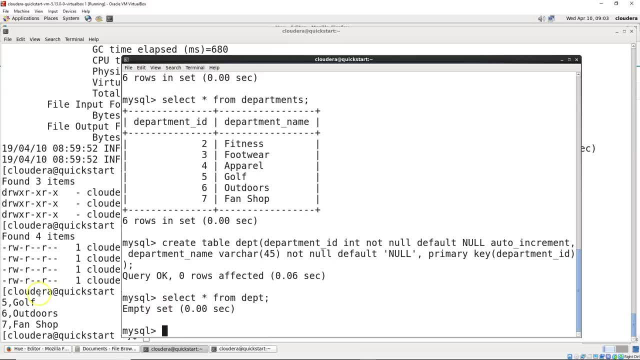 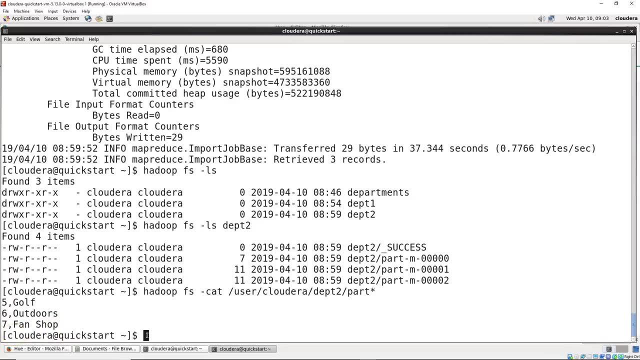 A new database, a new data table, and it's empty in there. So now we need to go ahead and export our data that we just filtered out into there. So let's flip back on over here to our scoop setup, which is just our Linux terminal window. 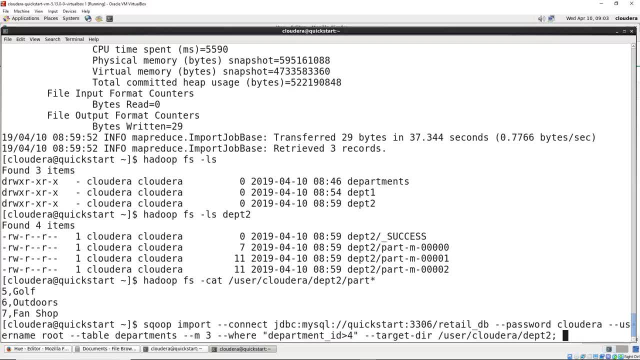 And let's go back up to one of our commands. Here's scoop, import. In this case, instead of import, we're going to take the scoop and we're going to export. So we're going to just change that Export, And the connection is going to remain the same. 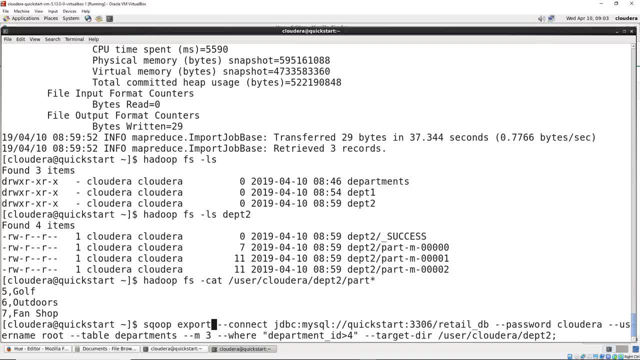 So same connect, same database. We're still doing the retail DB. We have the same password, so none of that changes. The big change here is going to be the table instead of departments. Remember, we changed it and gave it a new name. 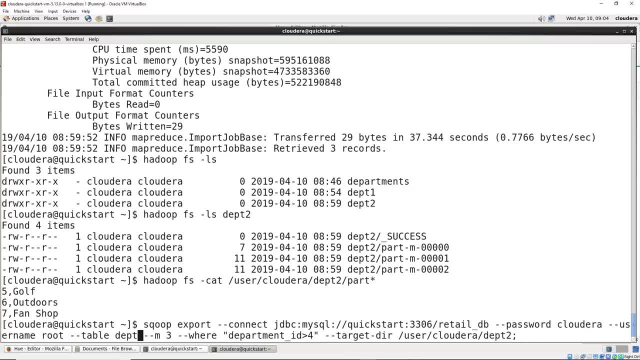 And so we want to change it here also: DEPT, So department, We're not going to worry about the mapper count And the where was part of our import. There we go, And then finally it needs to know where to export from. 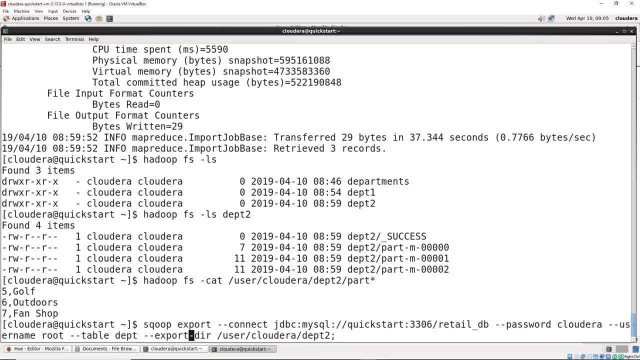 So instead of target directory, we have an export directory. That's where it's coming from- Still user Cloudera- And we'll keep it as department too, Just so you can see how that data is coming back that we filtered in. 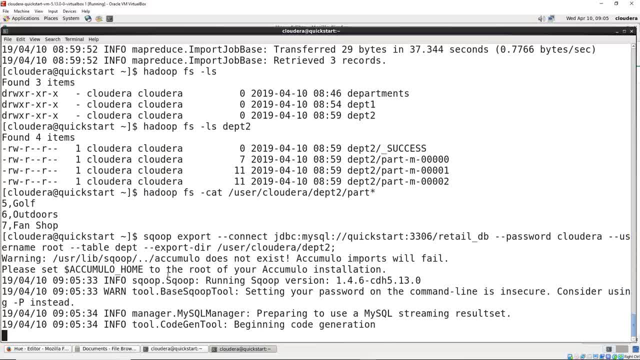 And let's go ahead and run this. It'll take it just a moment to go through its steps And again, because it's slow, I'm just going to go ahead and skip this so you don't have to sit through it. And once we've wrapped up, 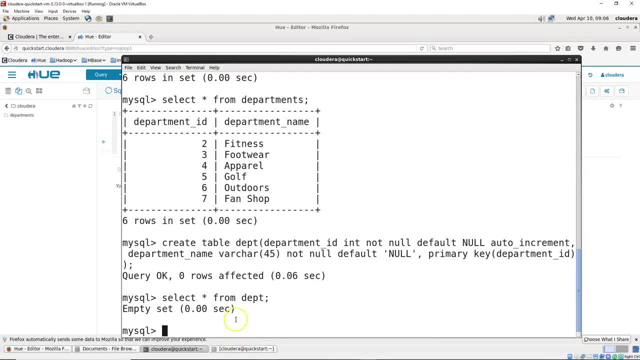 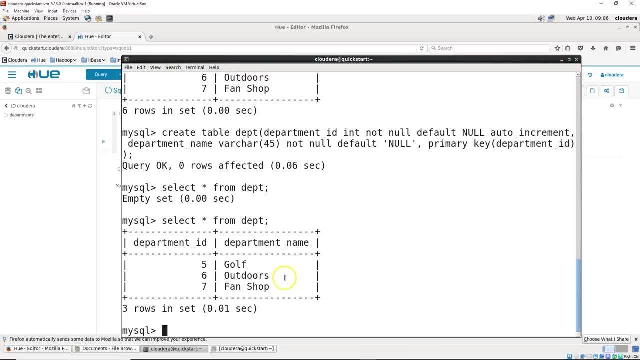 our export. We'll flip back on over here to MySQL, Use the up arrow And this time we're going to select star from department And we can see that. there it is. It exported the golf outdoors and fan shop And you can imagine also that you. 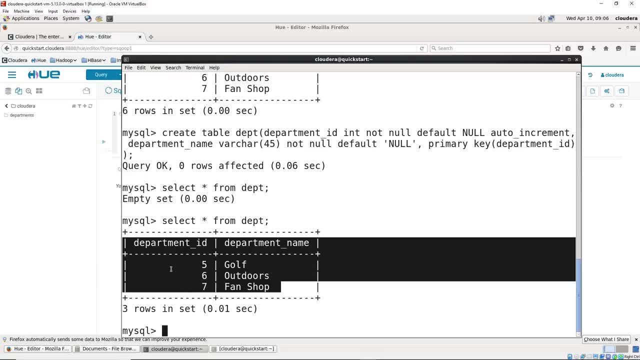 might have to use the where command in your export also, So there's a lot of mixing. The command line for scoop is pretty straightforward. You're changing the different variables in there, Whether you're creating a table listing a table listing databases. 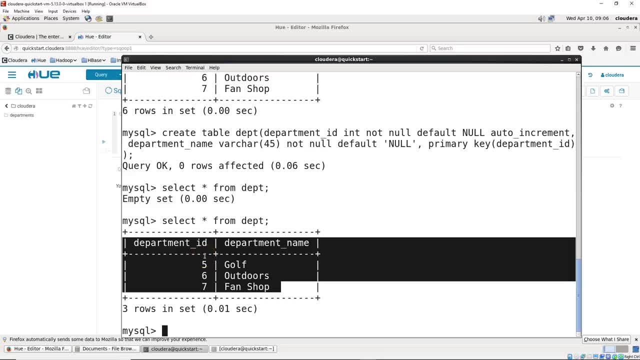 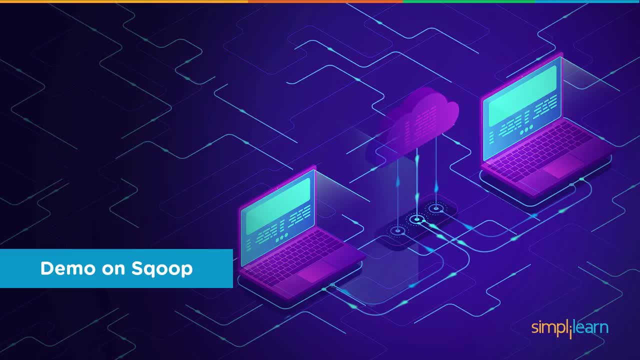 Very powerful tool for bringing your data into the Hadoop file system and exporting it. So, now that we've wrapped up our demo on scoop and gone through a lot of basic commands, That wraps it up for us today. I want to again thank you for.